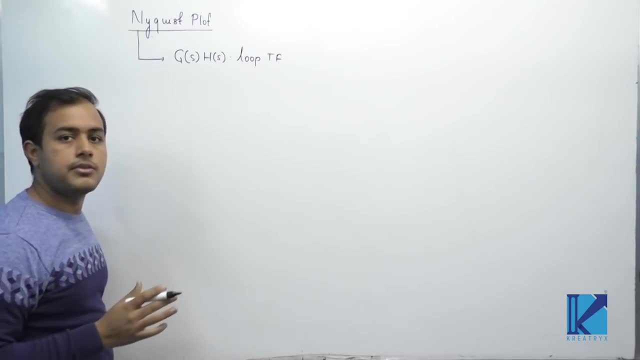 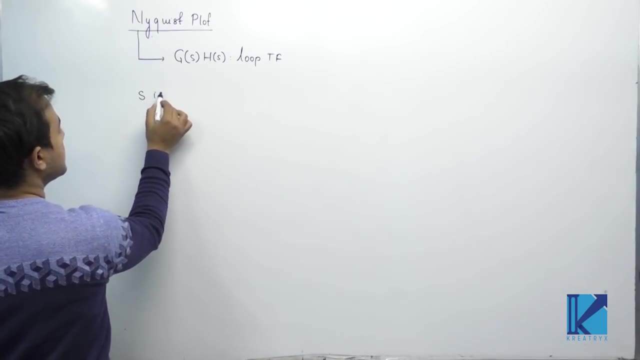 Okay, And it tries to map some value of S in the Gs Hs plane. What does that mean Actually, here? S is a complex number, right? S is a complex number. S is a complex number. S is a complex number which is expressed as S equal to sigma plus j, omega. 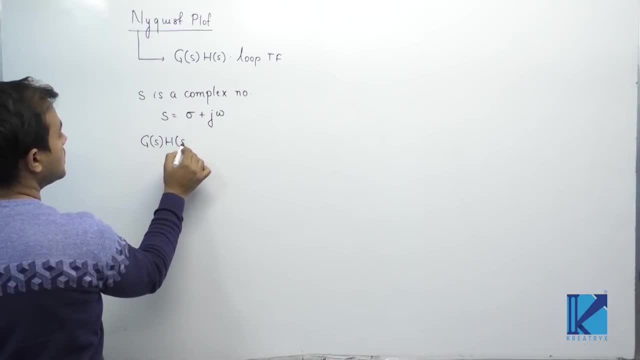 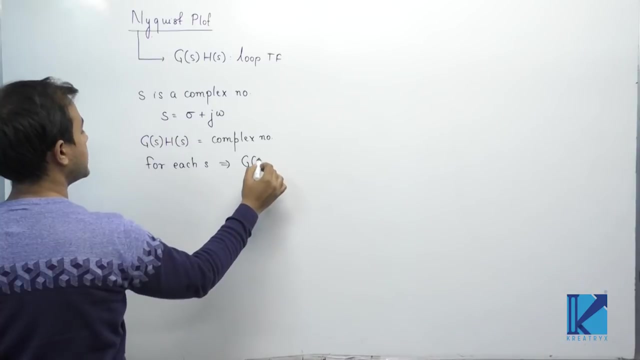 Then this Gs Hs. it is also a complex number. So basically for all, for each S we can define a value Gs Hs. That is, for different values of S, you can always find this value: Gs Hs. 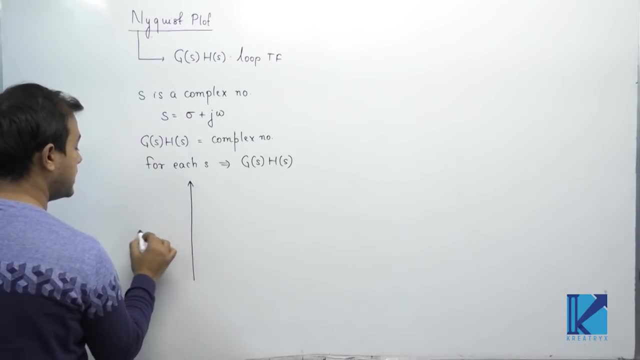 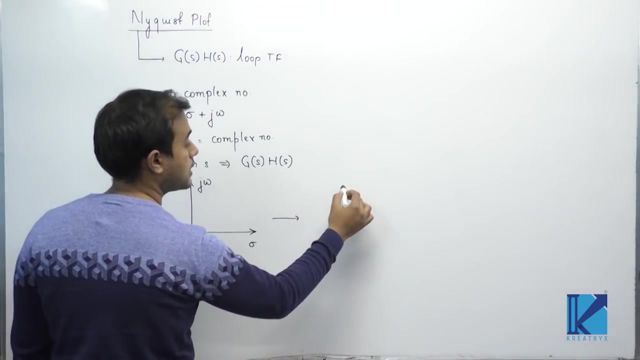 So what happens? we have two planes, basically. One is called as S plane. Here real X is sigma, imaginary X is j, omega. That is called as S plane, Okay. And there is another plane, another complex plane, that is called as GH plane. 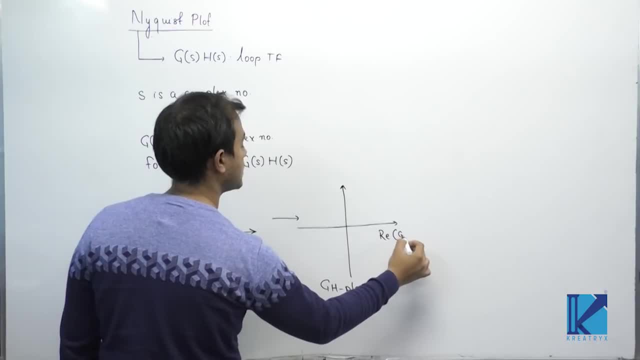 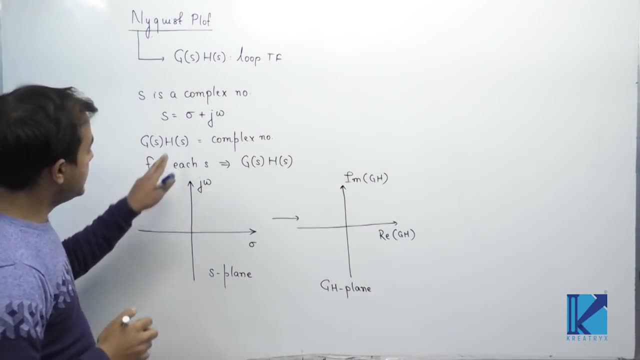 Here the real X is real part of GH And imaginary X is imaginary. Now, as I have already told you, that Gs, Hs is a complex number as well as S is a complex number, So we have two Xs, real and imaginary. 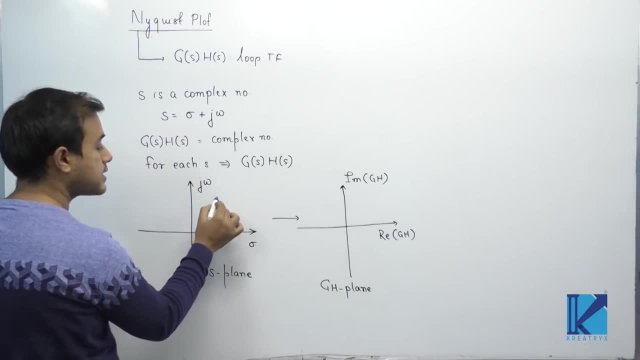 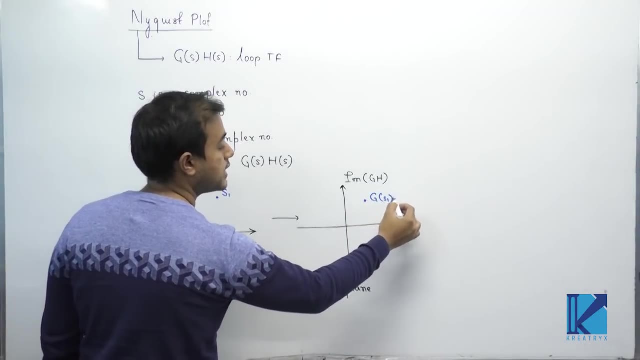 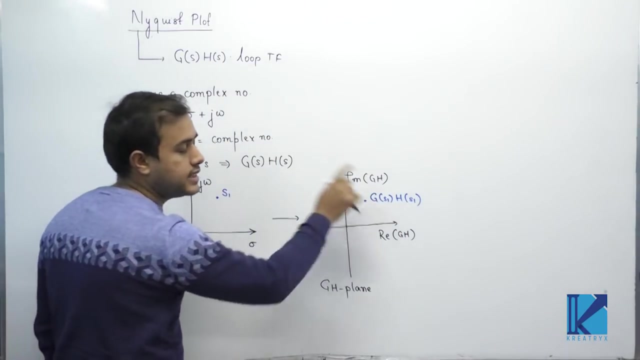 So what I want to do is, if I consider any value of S here- suppose S1,, there will be a corresponding point here, that is Gs1 into Hs. So I want to map certain points from the S plane to the Gs, Hs plane. 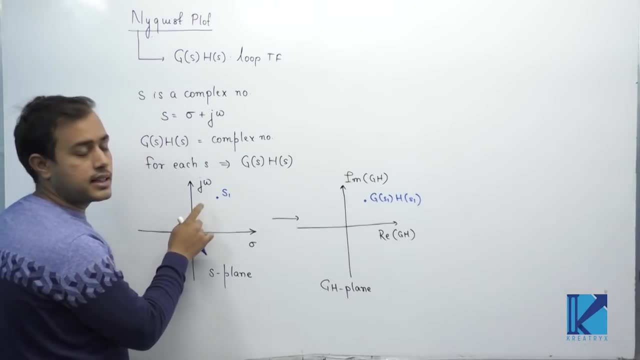 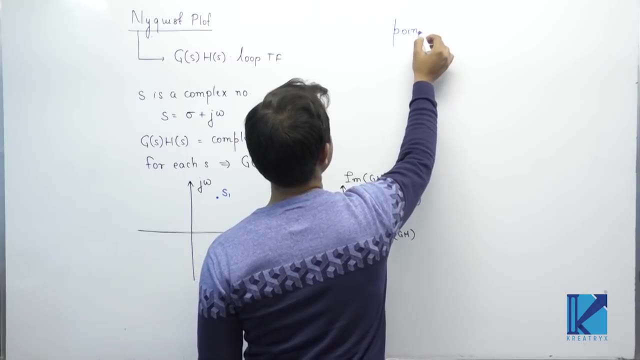 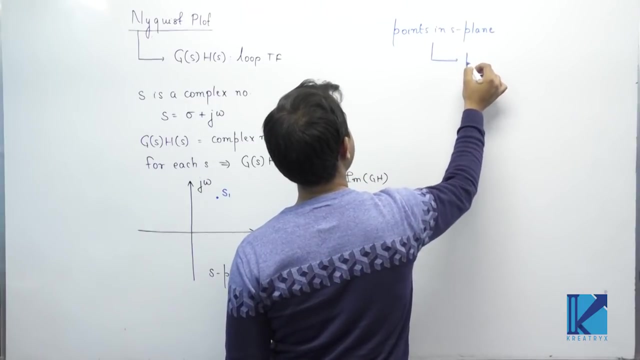 Now for that. I want to map certain points from the S plane to the Gs Hs plane Now for that purpose, first of all you will have to consider certain points in S plane. So whatever points in S plane you consider for which you want to find out the value of Gs Hs are said to lie on a curve which is called as Nyquist contour. 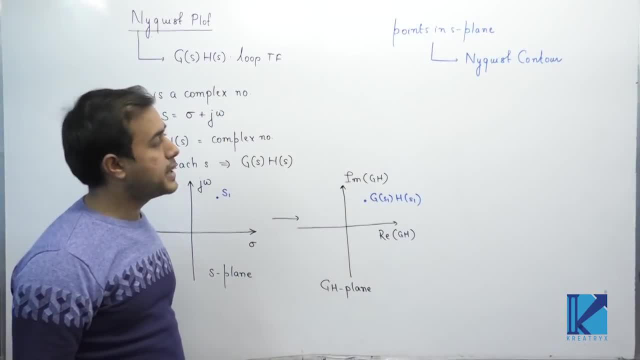 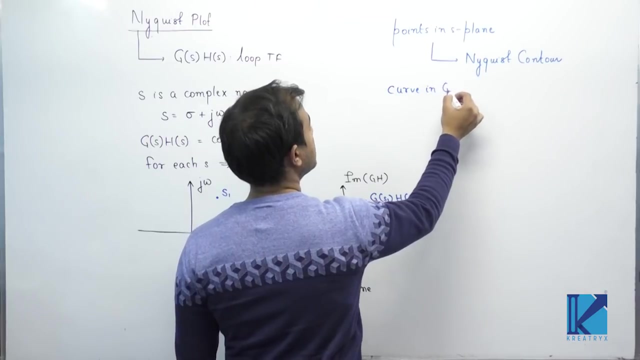 Okay So Nyquist contour is defined in S plane and it is a set of points, or the values of S, for which we will find out the value of Gs Hs. Okay So the curve in Gs plane, how you will get a curve in Gs plane. 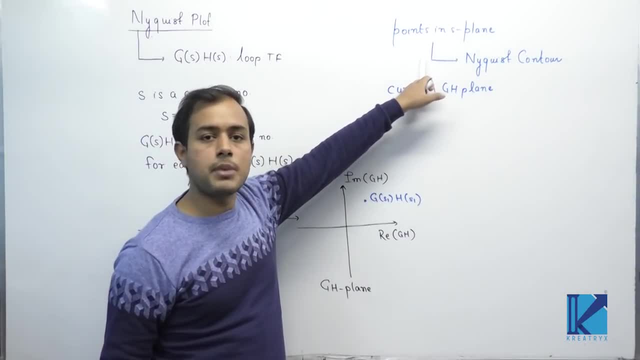 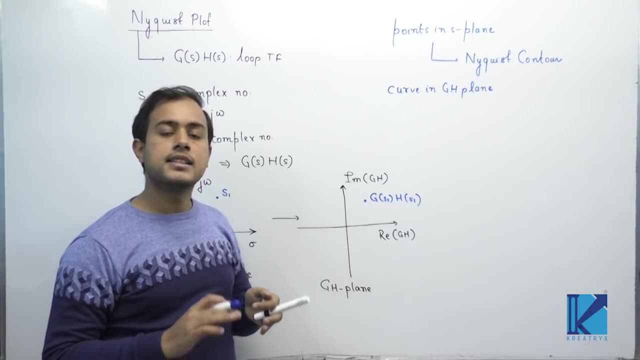 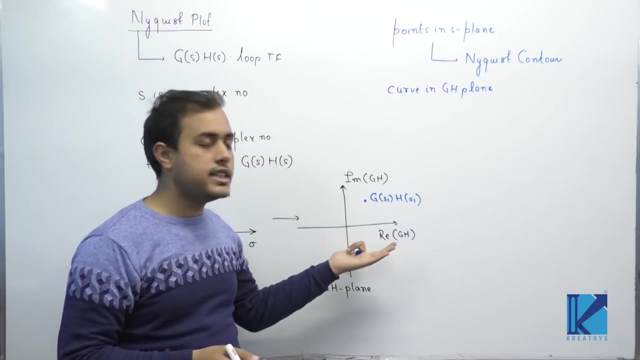 You will take some points in S plane or you take a points on a curve and corresponding points in Gs plane will also form a curve. What I mean to say? suppose, if you take a circle, If you take all values of S on a circle, you will get a corresponding image in Gs Hs. 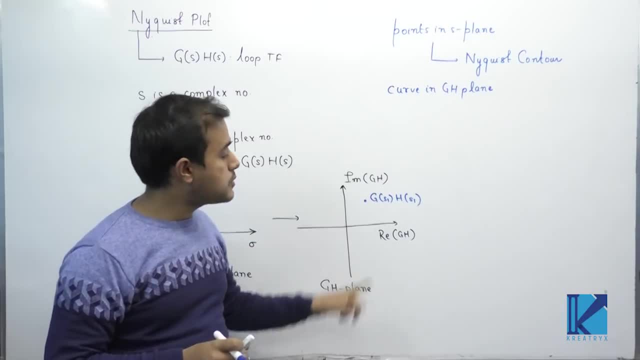 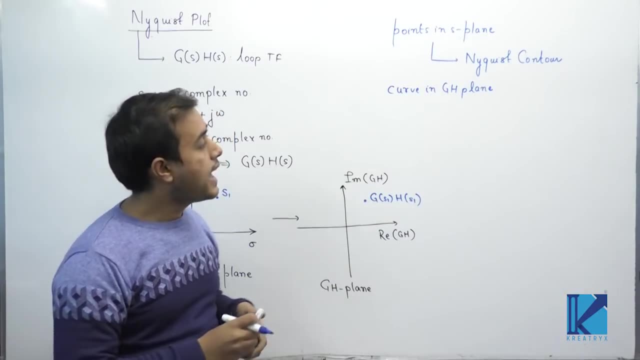 So how you do it. Suppose there are 10 points on a circle For each point, find this value and plot it on Gs plane. Keep plotting those points. They will also form a locus and that locus is called as Nyquist plot. 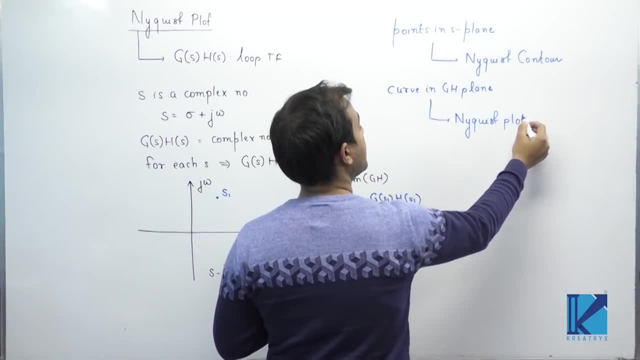 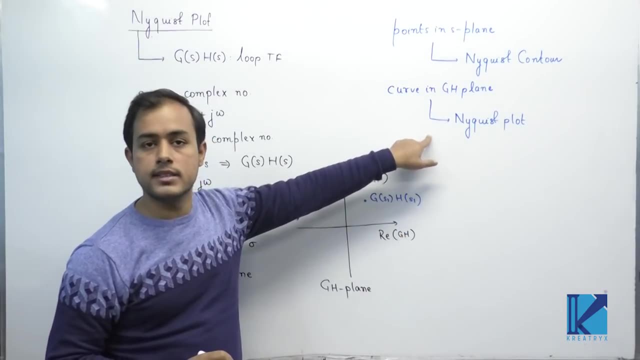 What I mean to say is: you take the values of S on Nyquist contour and corresponding values of Gs, Hs will lie on a Nyquist plot. So Nyquist plot will be drawn in Gs plane, whereas Nyquist contour will be drawn in S plane. 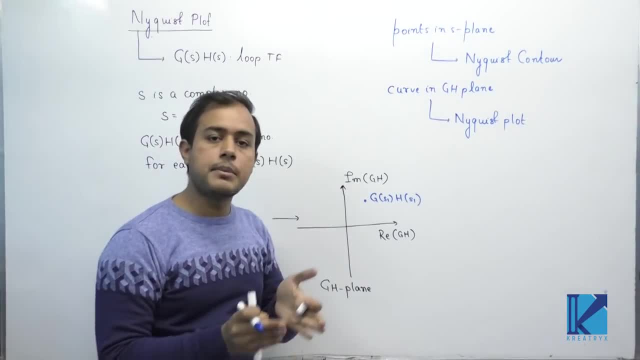 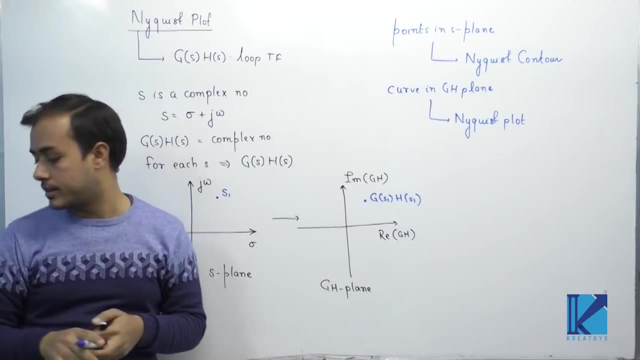 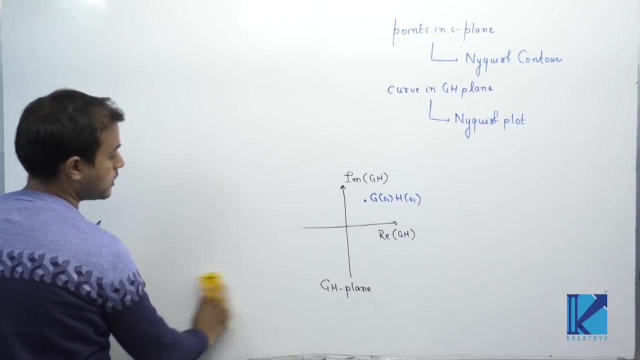 So it is nothing but Nyquist plot is a mapping of Nyquist contour on the basis of the function Gs, Hs. So it is nothing, but it is a mapping. Now, first of all, what we do is, first of all, we have to define a Nyquist contour. 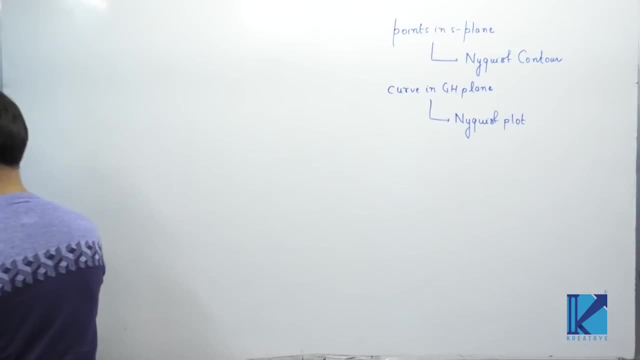 Okay, So let me define a Nyquist contour. Nyquist contour is taken as the entire right half plane. A curve which should enclose the entire right half plane is taken as the Nyquist contour. Okay, So how we take it. 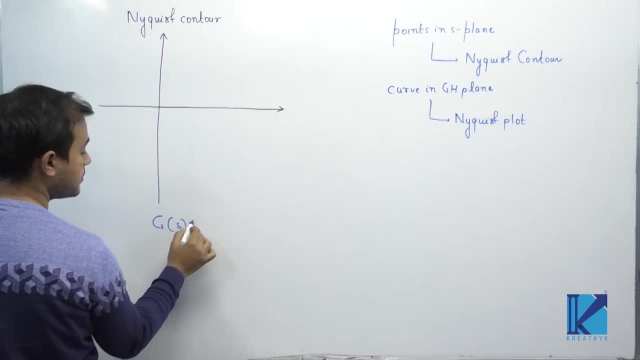 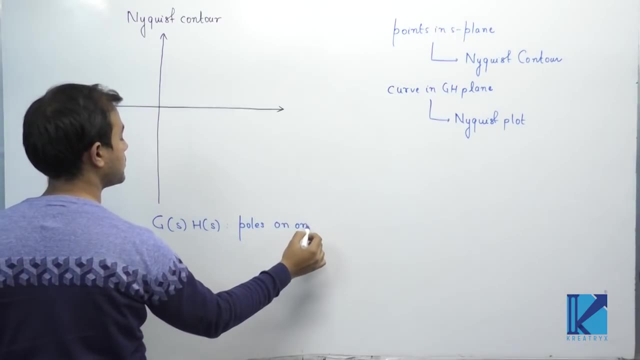 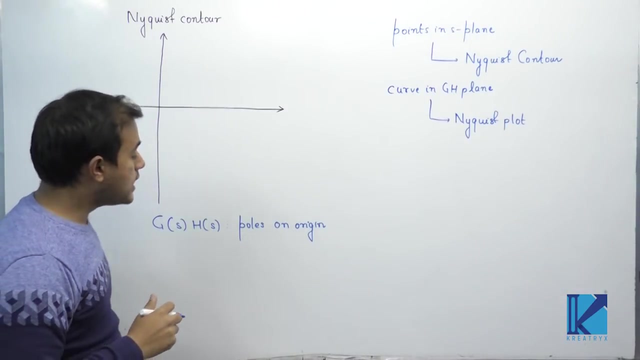 Suppose Gs, Hs is a transfer function, basically It will have certain poles. Suppose there are poles on origin. Now poles are the points where the value of function is undefined. So you can understand I can never substitute the value of pole in this function. 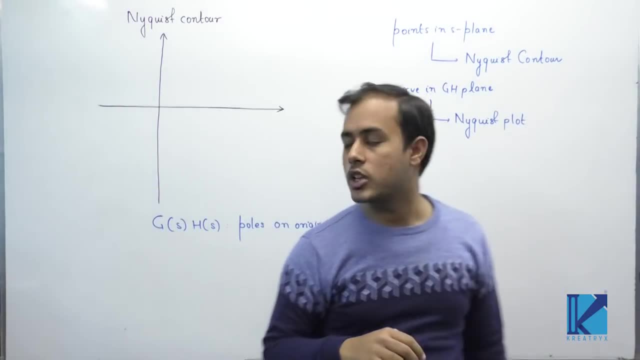 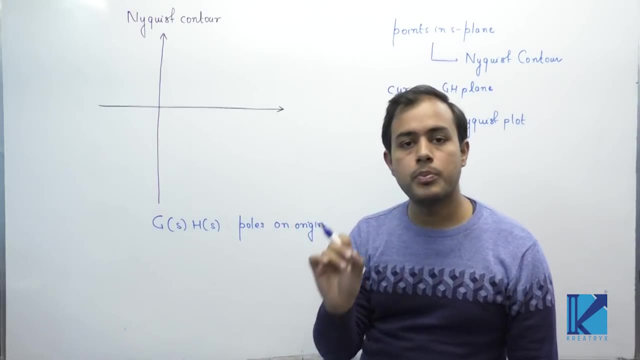 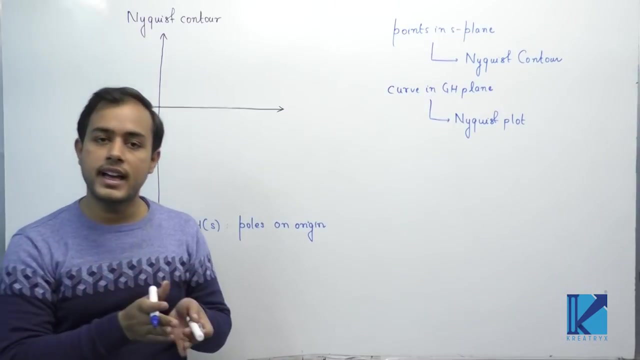 Because if you substitute the value of pole, the value that you will obtain will be undefined. That is what. On the Nyquist contour, there should be no pole of Gs, Hs, Because Nyquist contour is nothing, but it is a set of values of S that you will substitute. 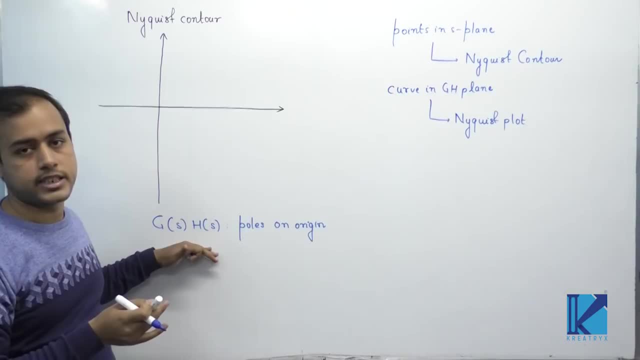 in this function to obtain the values of Gs, Hs. Okay, So on Nyquist contour, there should be no pole of this transfer function. Now suppose this transfer function has a pole on origin. So when you are taking a Nyquist contour, you will have to take it in such a way that 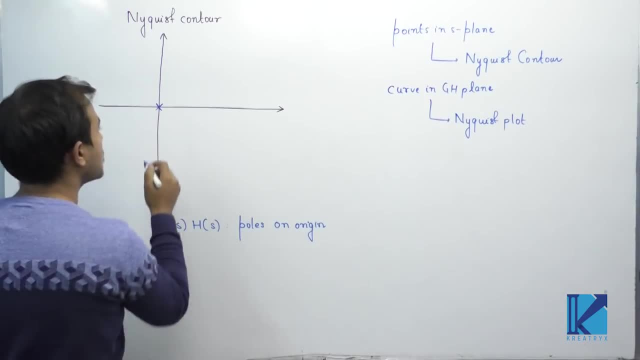 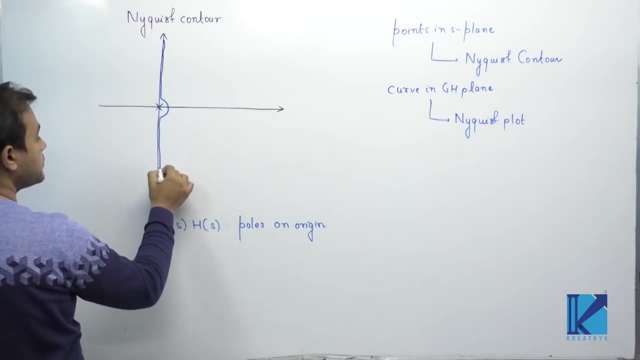 you avoid this. You have to avoid this origin. So see how you will do it. We take a Nyquist contour like this: Okay, So there is entire right half plane inside this and the direction is like this: Okay, It is a closed curve. 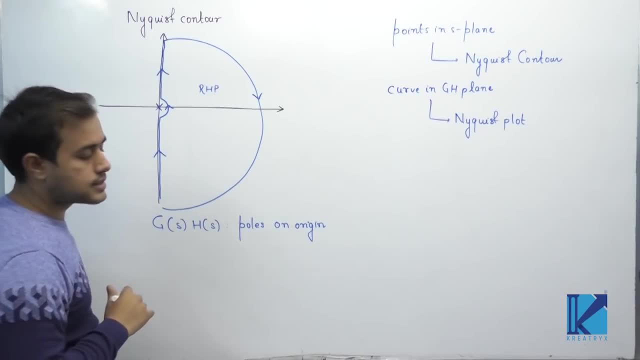 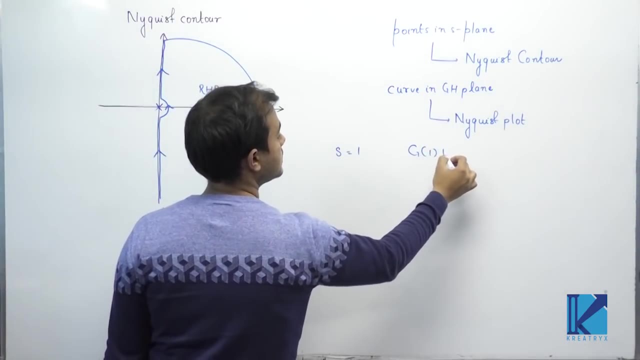 Closed curve implies we will end at the same point where we all started. So see, Suppose you started S equal to 1.. The value that you will get is G1.. H1.. If you end also at S equal to 1, you will again get the value G1. 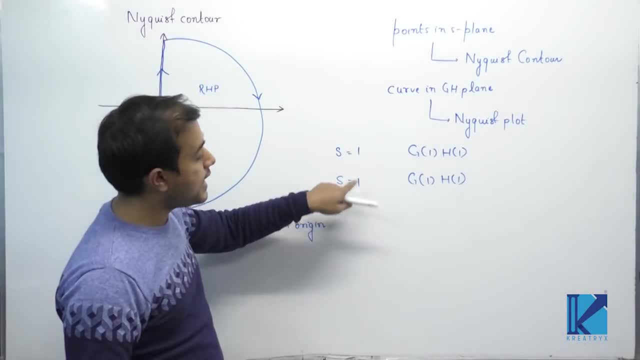 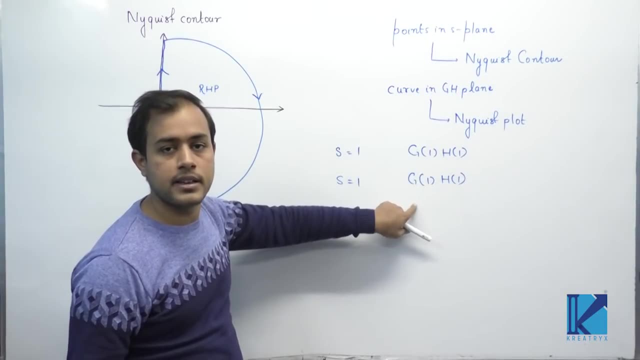 H1.. Which means if you start and end at the same point in S plane, you will start and end at the same point in Gs Hs Plane, Which means a closed curve in S plane will always give a closed curve in Gs. 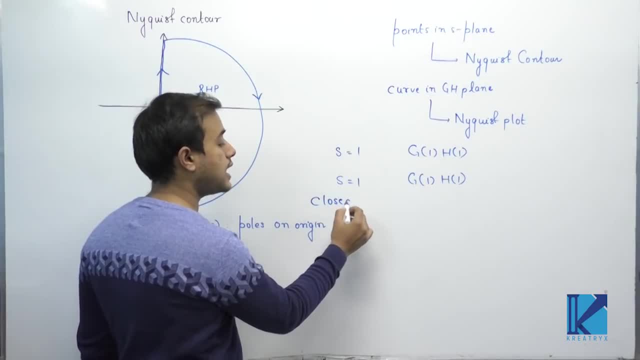 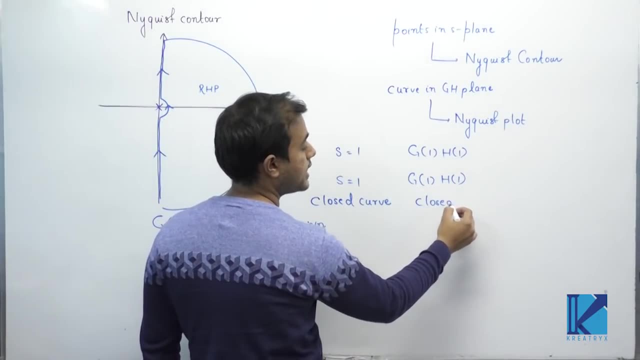 Hs Plane. Is it fine? If you start and end at the same value of S, you will start and end at the same value of Gs, Hs. So a closed curve in S plane is mapped to a closed curve in Gs. 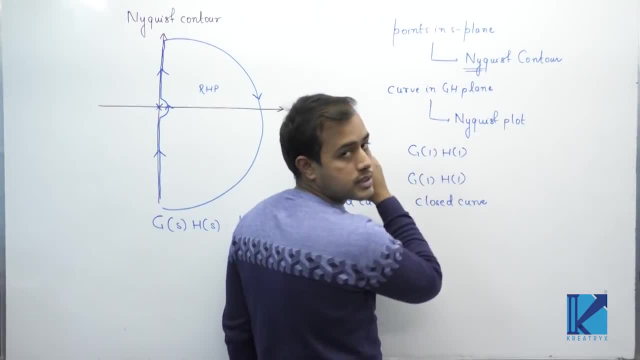 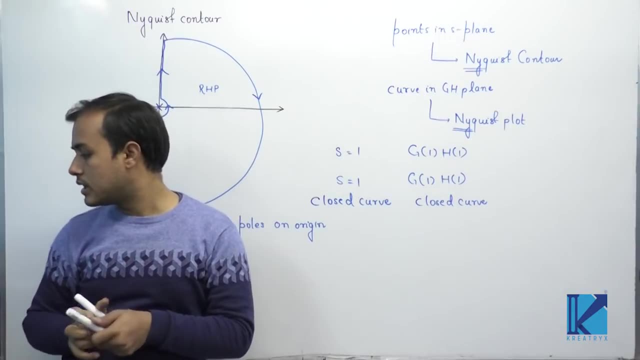 Hs Plane. So Nyquist contour is also a closed curve. Nyquist plot is also a closed curve. Both curves will start and end at the same point. Now, in order to find out the value of Gs, Hs. 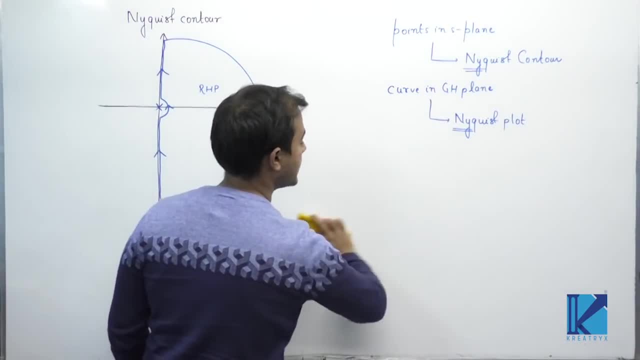 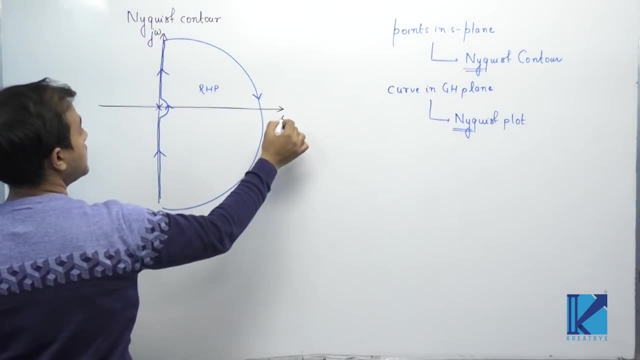 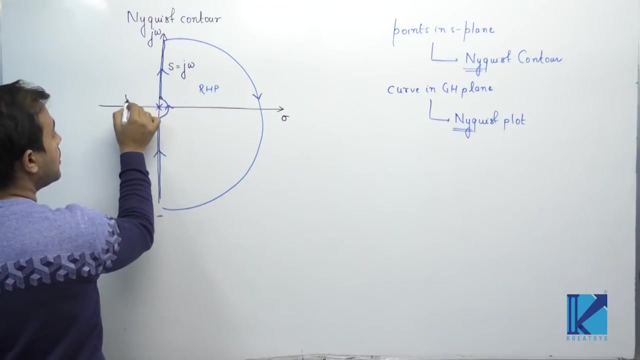 First of all we will divide the Nyquist contour into certain points, Into certain parts. So this first part, Here, basically S, is imaginary. So here we keep S equal to j, omega. Here omega will go from omega equal to 0 up to omega equal to infinity. 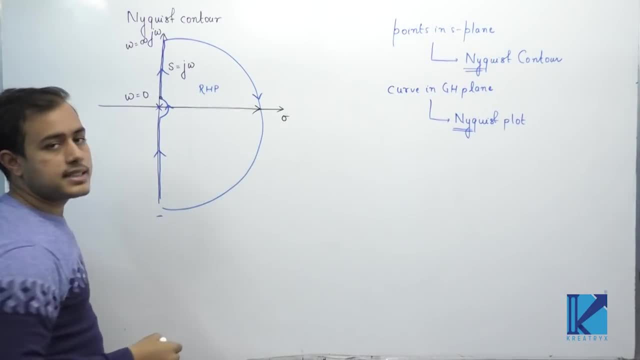 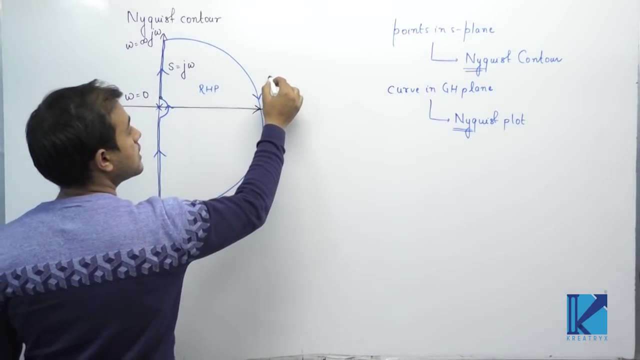 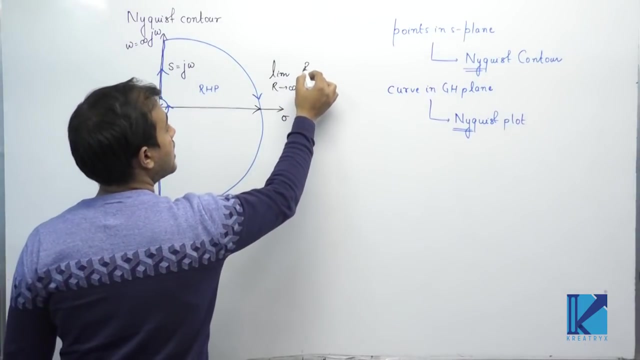 Okay, This one. This is the infinite semicircle, so that it encircles or encloses the entire right half plane. How do we do that? Simply limit R tending to infinity, That is, the radius tending to infinity. R e to the power j theta. 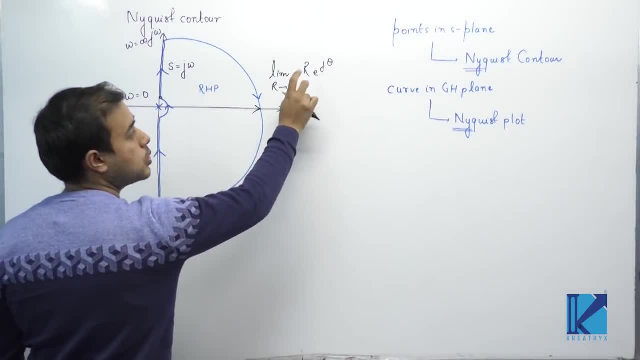 Okay, That is the equation of a circle whose radius is infinite And if you see, it is a semicircle. Here the angle is plus 90.. And here the angle is minus 90. So I can say the angle varies from plus 90 to minus 90.. 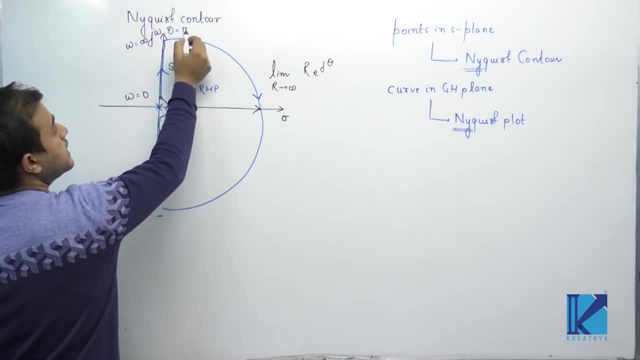 I can also say the angle varies from minus 90 to minus 90.. I can also say that you will find this angle surrender to a value of 0. You can also see that this angle does not look like a 0. So your angle is not look like an 0. 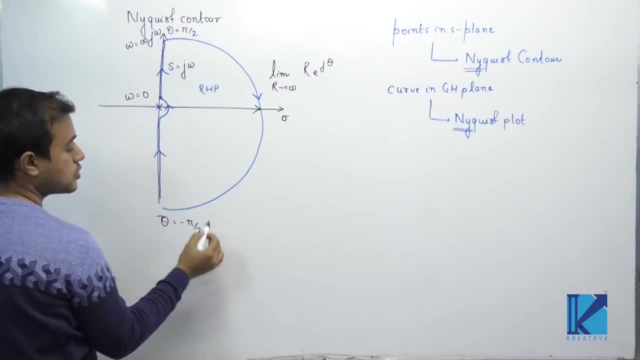 This angle is not look like a 0. Just imagine, And again, the angle is a 0. Because you see, our angle is 0. This angle is 1.. varies from plus 90 to minus 90, okay, Then this one. this is a negative imaginary axis. 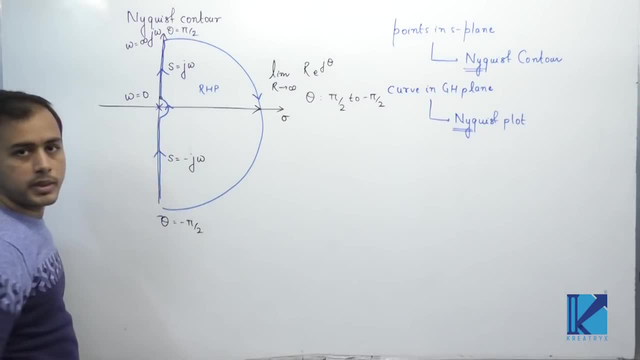 so s will be equal to minus j omega. and then this is a very small semicircle which is used to avoid the origin, So r e to the power j theta, where r tends to 0.. This is again a semicircle whose radius is tending to 0., But here theta is going from minus 90 to. 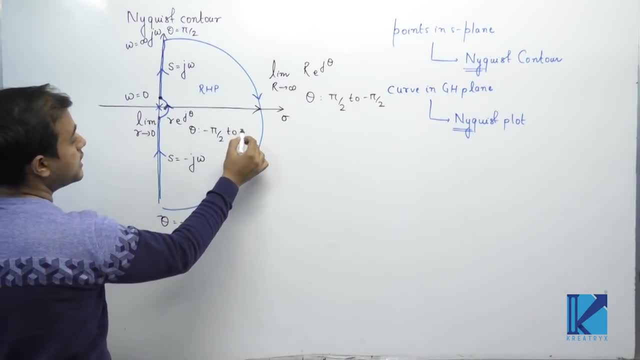 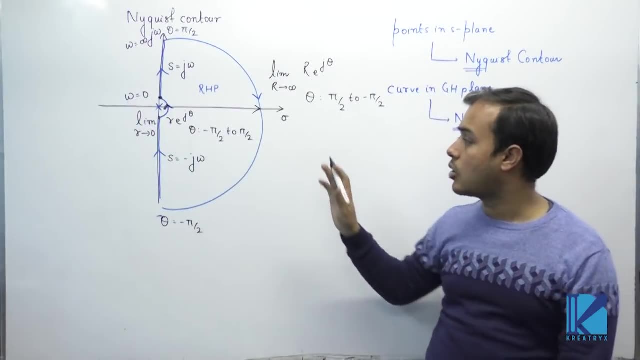 plus 90. So theta from minus pi by 2 to plus pi by 2.. So these are the four parts of a Nyquist contour. We take care that we do not encircle or do not. sorry, we do not. 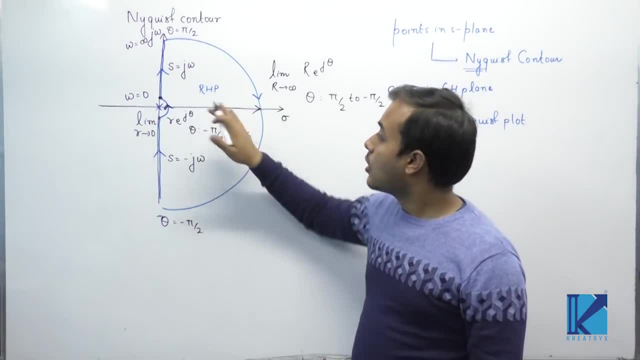 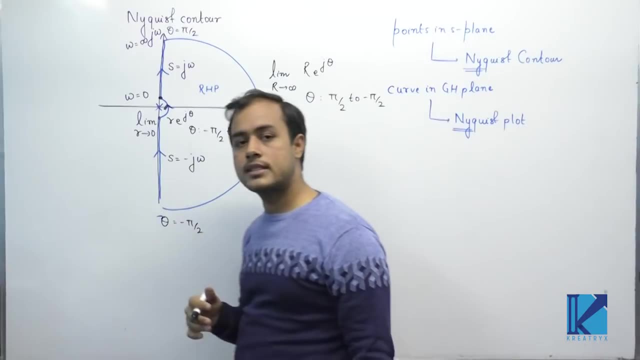 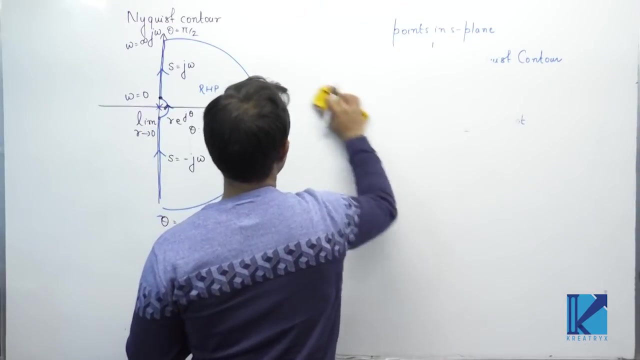 pass through any pole of GSHS, because all these values of s will be substituted in the function GSHS in order to draw the Nyquist plot. Now let me show you how you find out the Nyquist plot. So let me mark these curves. 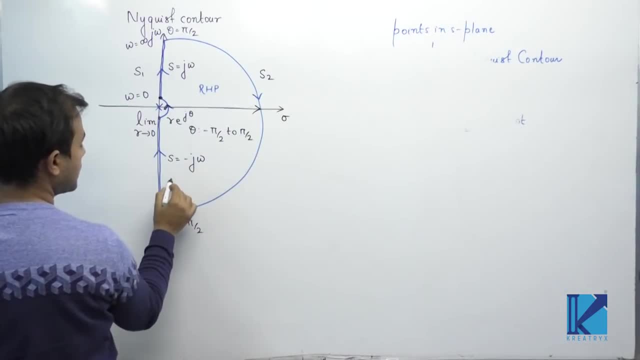 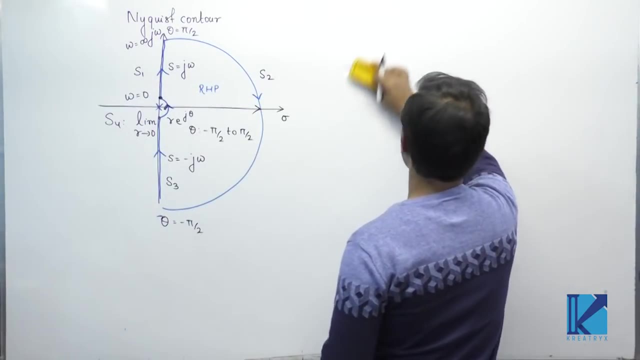 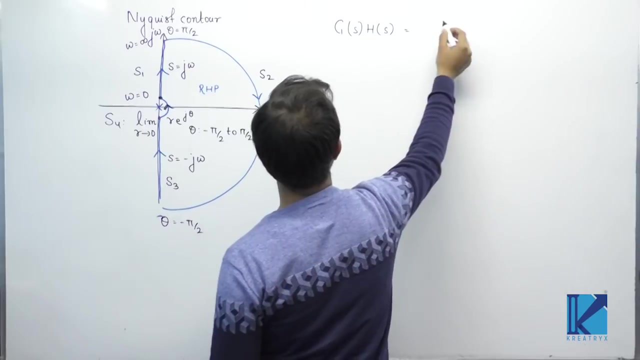 as s1, s2, s3, s4.. There are four parts in this Nyquist contour, So let us take one transfer function. in order to understand GSHS, Let me take 1 upon s, 1 plus s, 1 plus s. 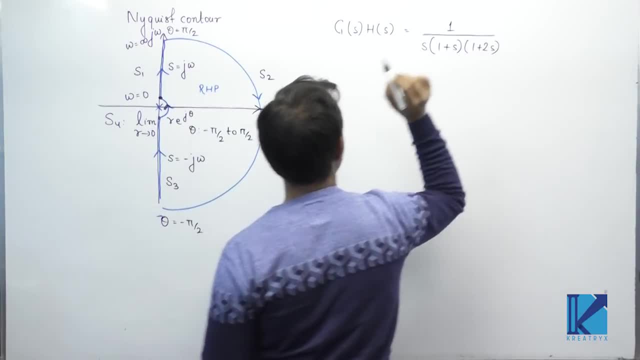 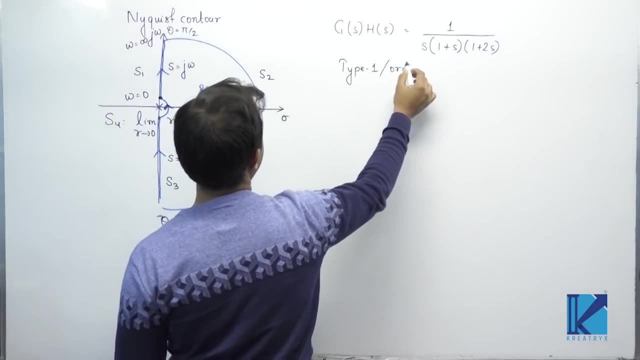 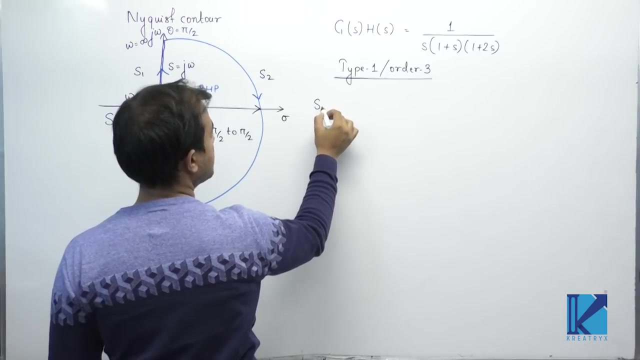 1 plus 2s. This is the most common type of transfer function that is asked in GATE. It has type 1 and order 3.. It is very common in GATE example. So first let me find out the value of GSHS for s1.. For s1, you will keep s equal to j omega, So it will be gj. 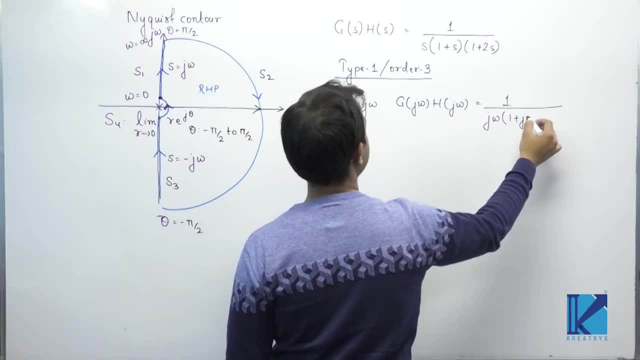 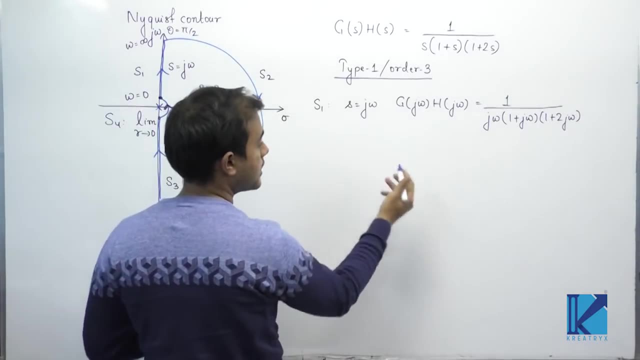 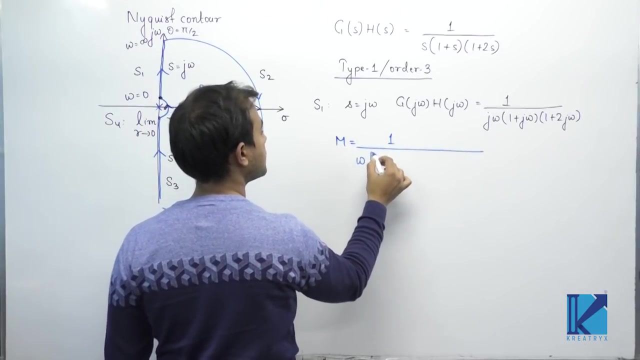 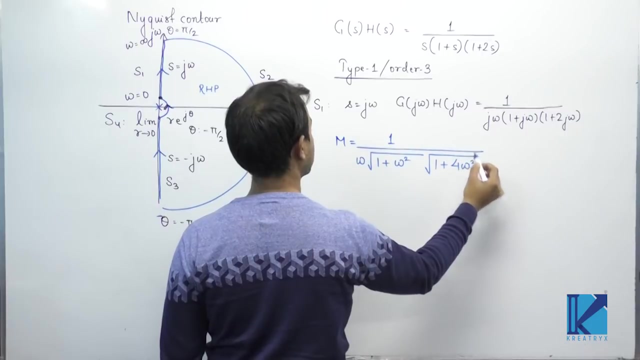 omega: 1 plus j omega and 1 plus 2j omega. So basically here what you do is you find out two values. One is the magnitude. What will be the magnitude? Omega under root: 1 plus omega square. under root, 1 plus 4 omega square. Second one is the phase. I am assuming 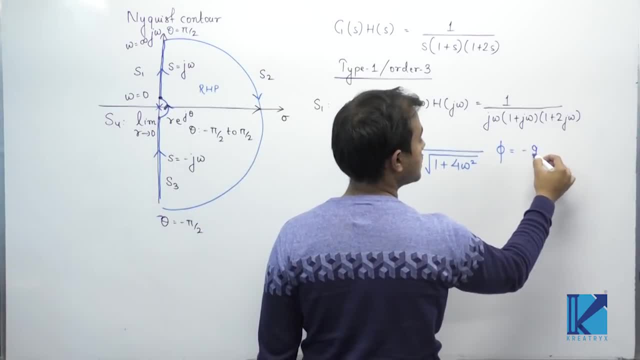 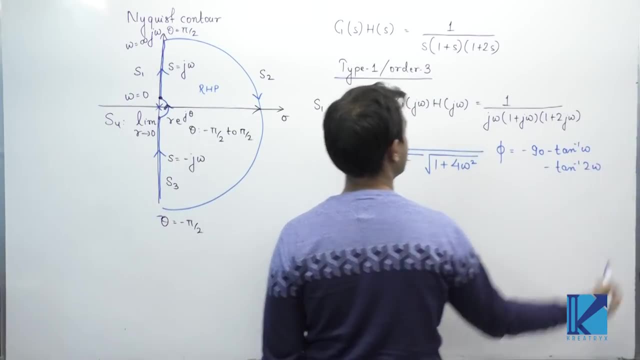 that you know how to derive this magnitude. So let me show you how to derive this magnitude. What is the magnitude and phase for complex number? Minus 90 minus tan inverse omega minus tan inverse 2.. That is the magnitude and phase. Now, as I told you, omega varies between 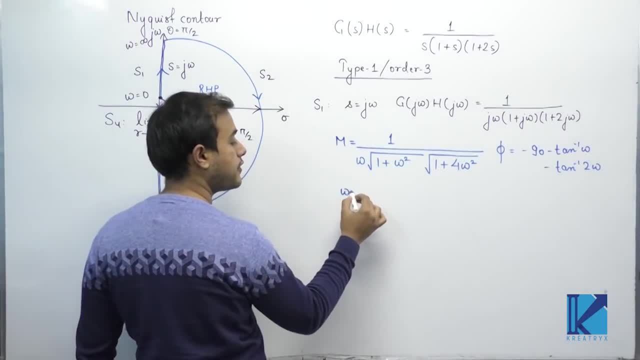 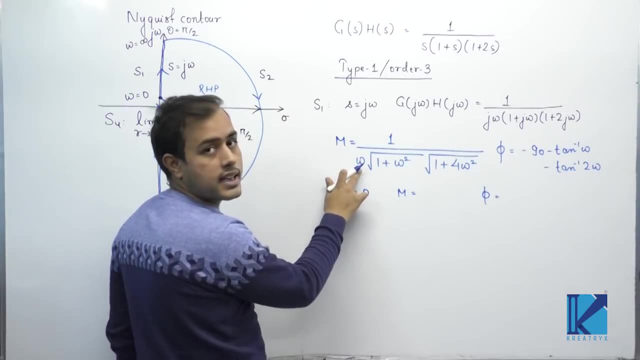 two values: 0 and infinity. So what we will do is we will find out the values of magnitude and phase at 0 and infinity. So, as you keep omega equal to 0,, this magnitude would be infinite. Omega equal to 0, tan inverse would be infinite. So, as you keep omega equal to, 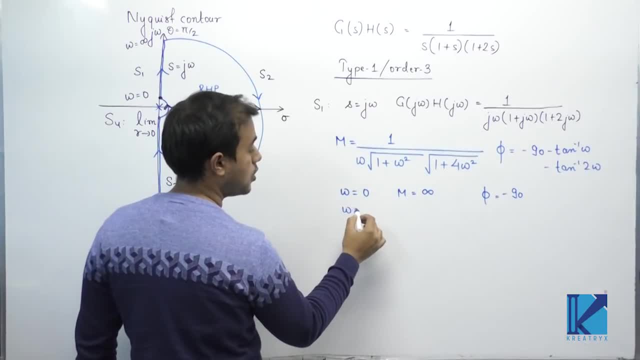 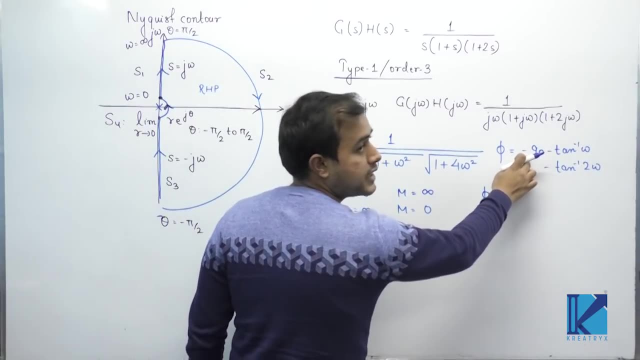 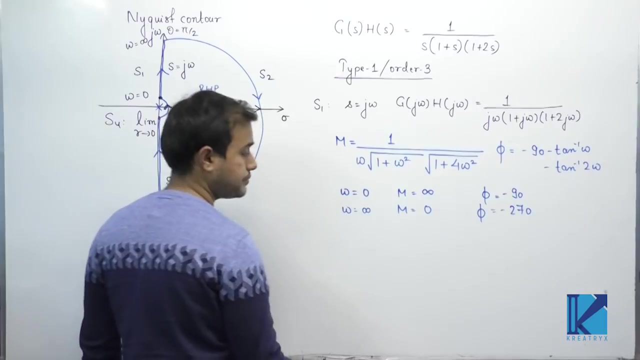 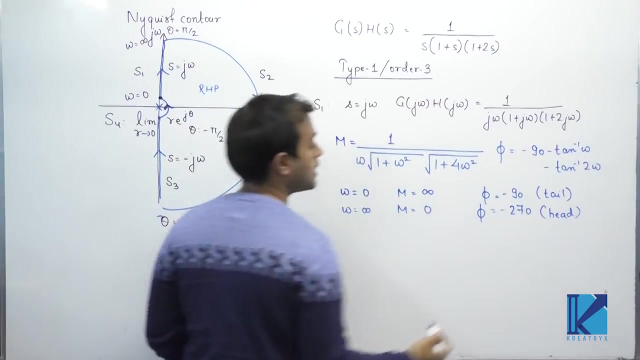 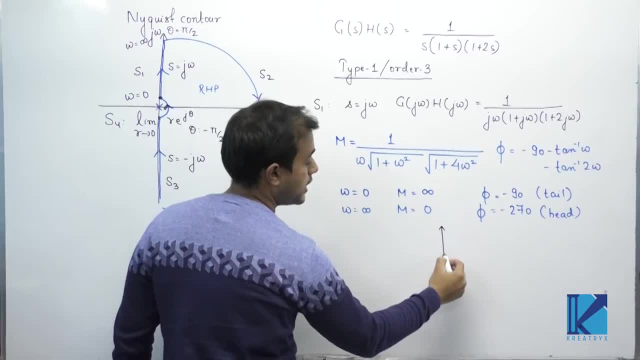 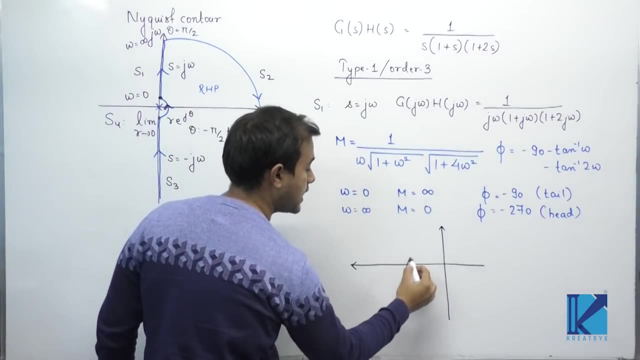 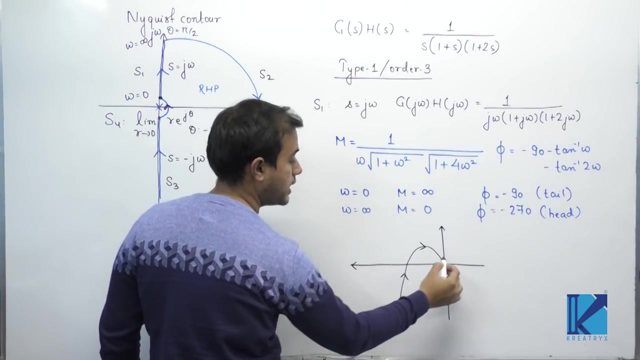 as you draw this curve here, the angle is going from minus 90 to minus 90.. So this is going to be minus 270, and magnitude from infinity to 0. So the curve is something like this: Okay, Here omega is 0.. Here omega is infinite. So this is called as the tail. 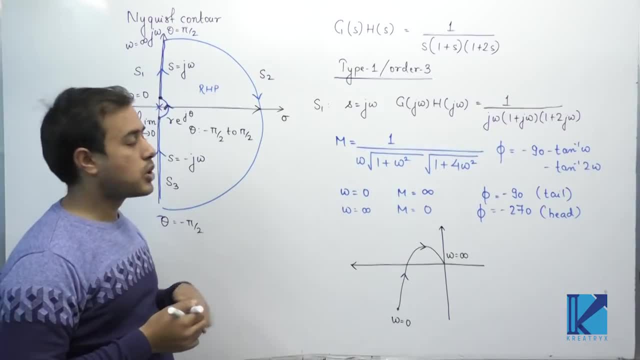 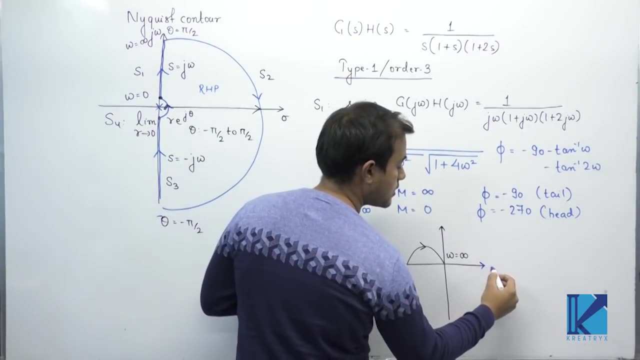 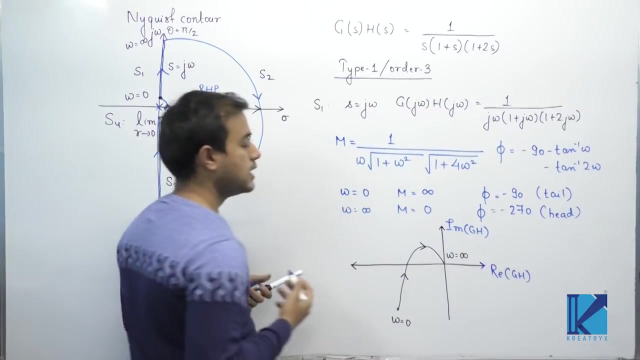 and this is called as the head. So I have basically plotted this one S1, from S plane to GSHS plane. Here the x's are real part of GH And this one is imaginary part of GH. So what I have done is I have taken every possible. 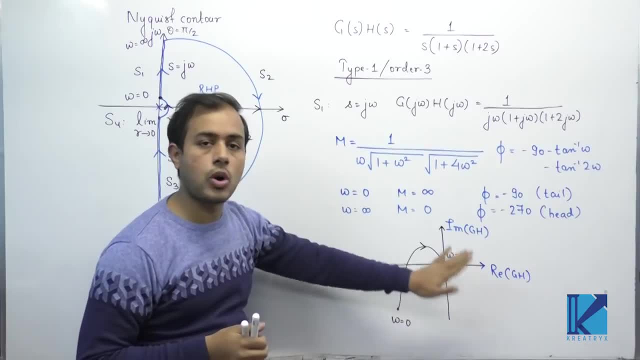 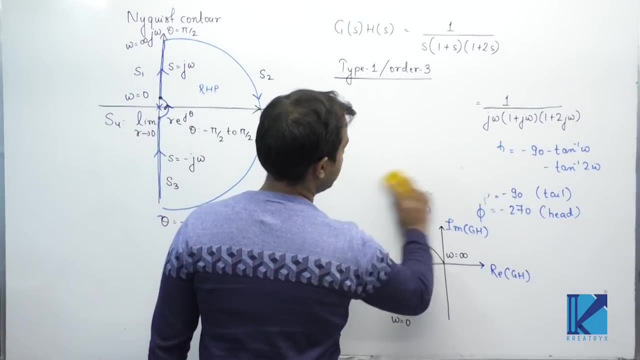 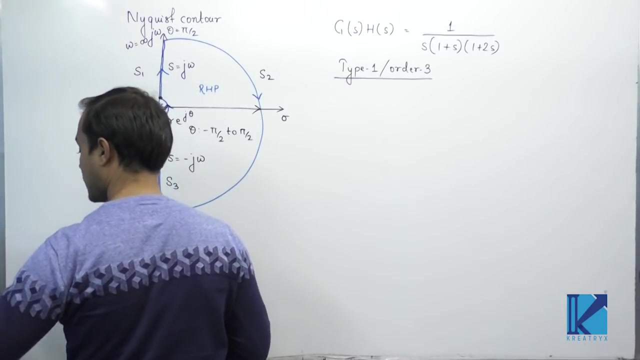 value of S, which is equal to J, omega, and find out all the values of GSHS. Okay, Understood this much. Next, let us come to the curve, S2.. Okay, Let us derive the Naive's plot for S2.. In case of S2, what you will do, Limiting 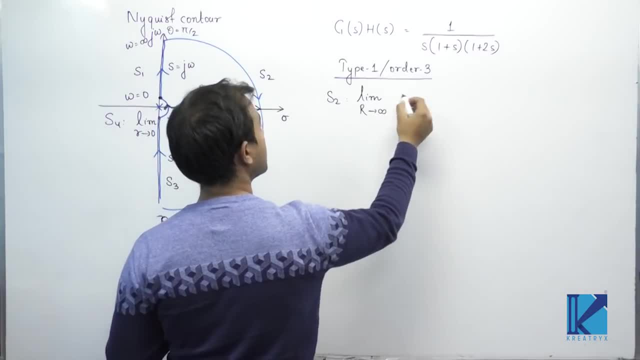 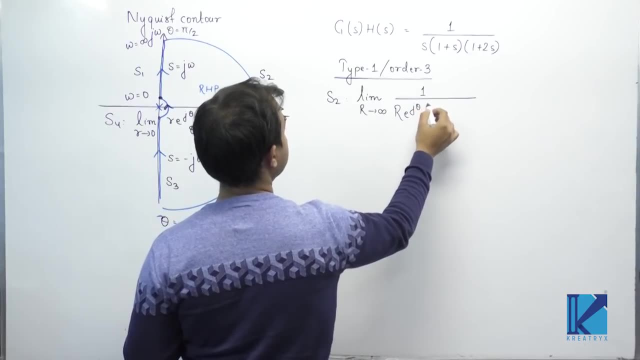 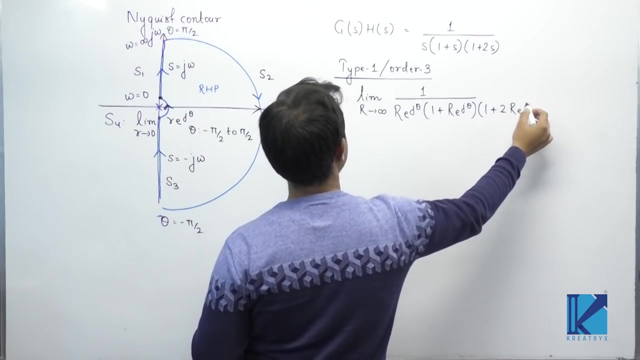 R tending to infinity, what you will do. 1 by I am substituting the value of S, 1 plus r? e to the power j theta 1 plus 2r e to the power j theta. Now, since r is much, much greater. 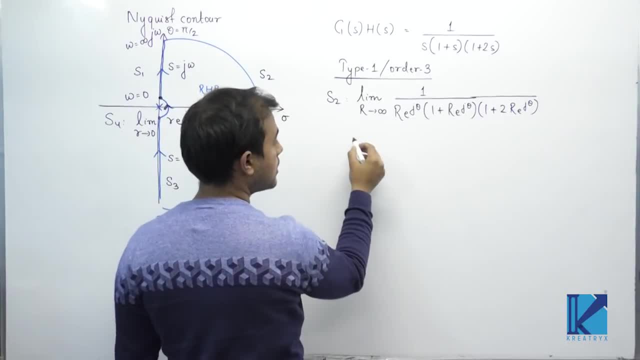 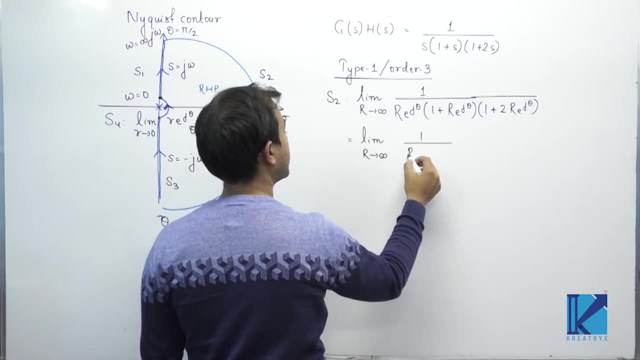 than 1, it is tending to infinity. I can ignore this one, So it will come out to be limiting. So this will be 1 upon r cube e to the power j, 3 theta. So this will turn out to be 0,. 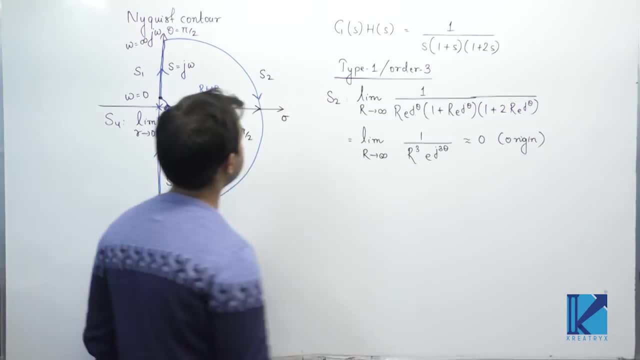 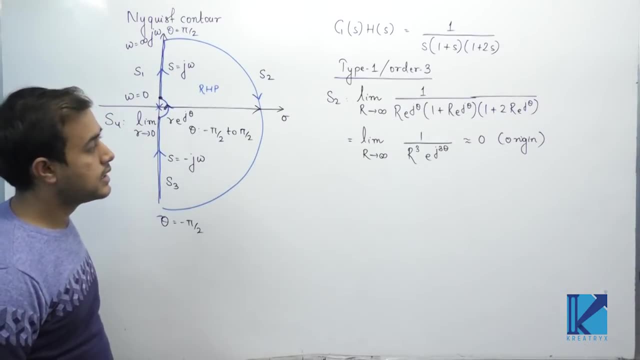 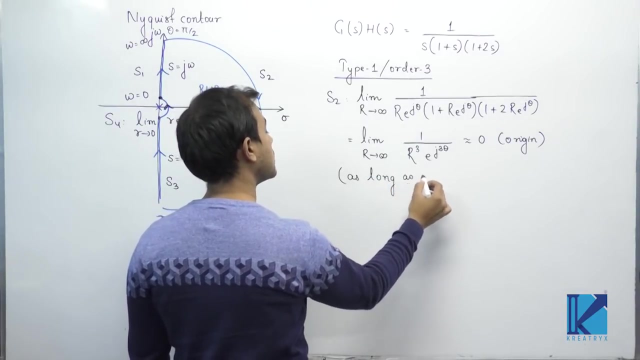 that is origin. So you do not have to worry about this infinite semicircle. It will be mapped to origin in the GSHS plane. It will simply be the origin. So how long this is valid? As long as order of denominator. 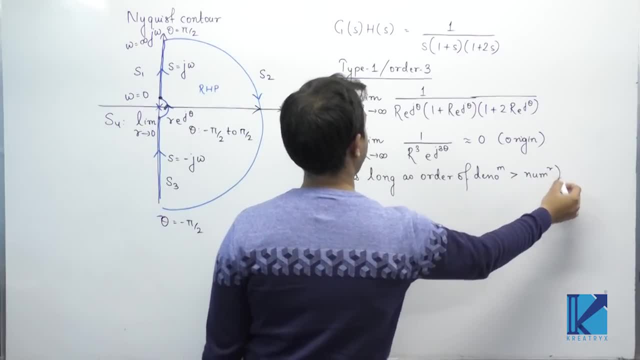 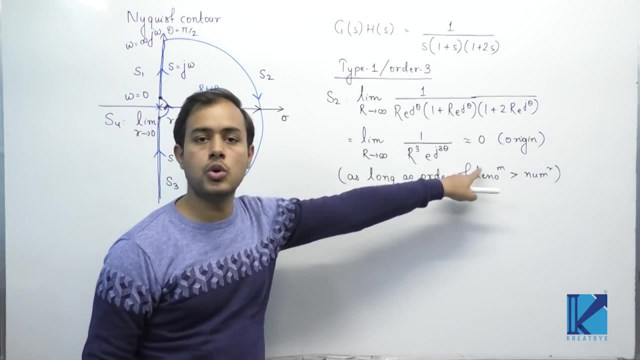 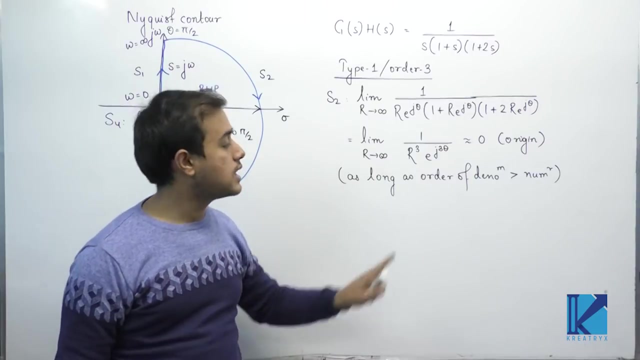 Is greater than numerator. Okay, If denominator has higher order, polynomial, as compared to the numerator, it will always map to origin. If the numerator had higher order than denominator, it will not be a proper transfer function. For proper transfer function, this condition. 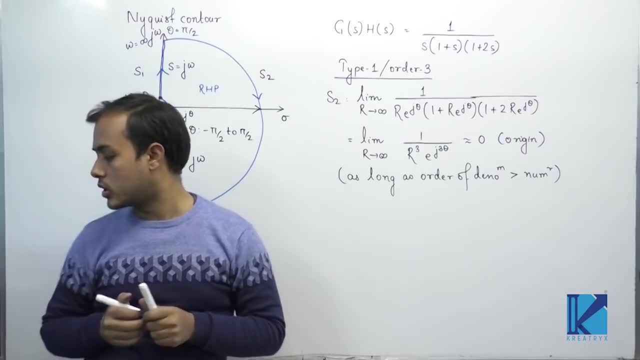 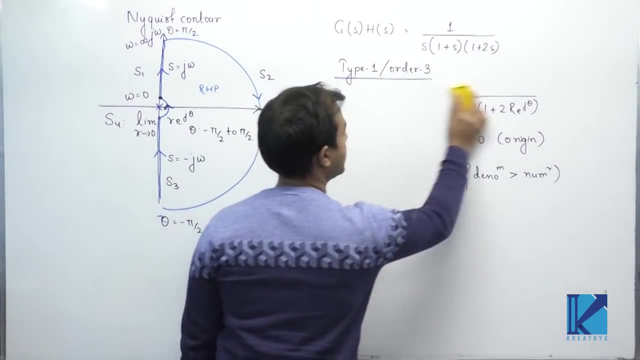 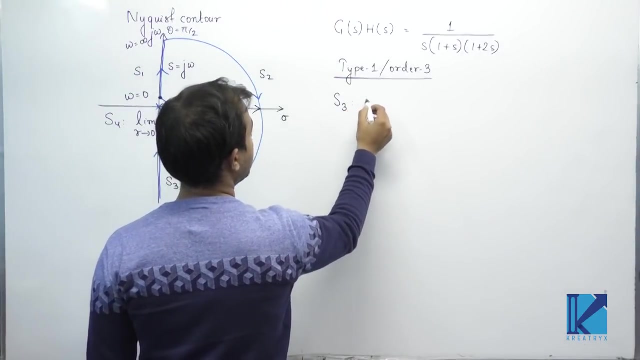 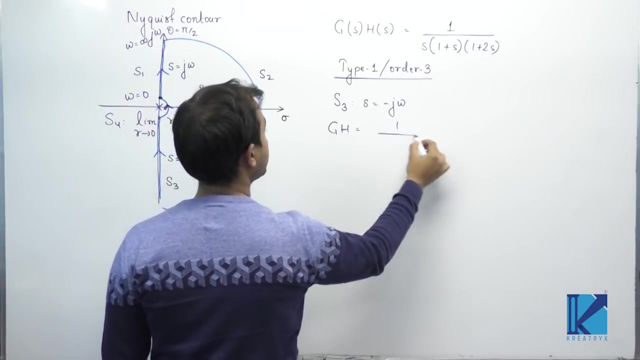 is the necessary condition: order of denominator greater than order of numerator. Now, what happens? Now let us map the next point, that is S3.. So in S3, what happens? You keep S equal to minus j omega, Which means GH will come. 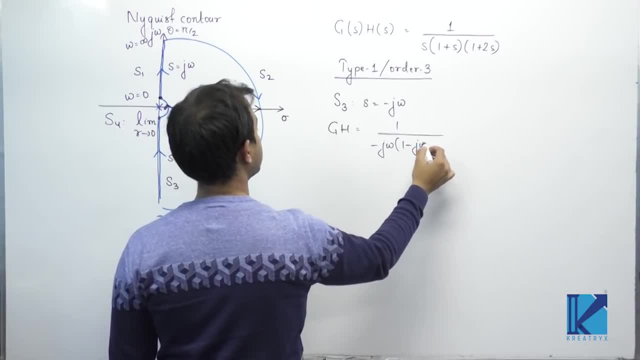 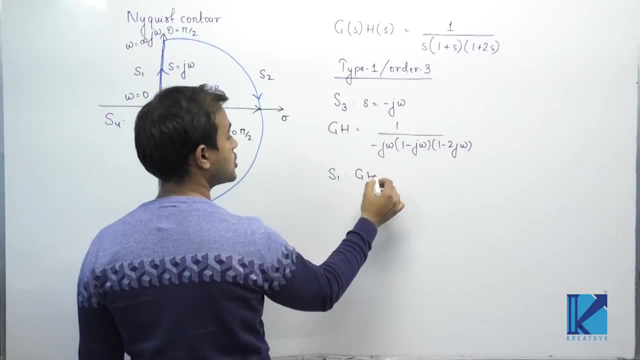 out to be 1 by minus j omega, 1 by minus j omega, 1 by minus 2 j omega, Earlier for S1, what was GH? 1 by j omega, 1 plus j omega, 1 minus j omega. So it is 1 by minus j omega. 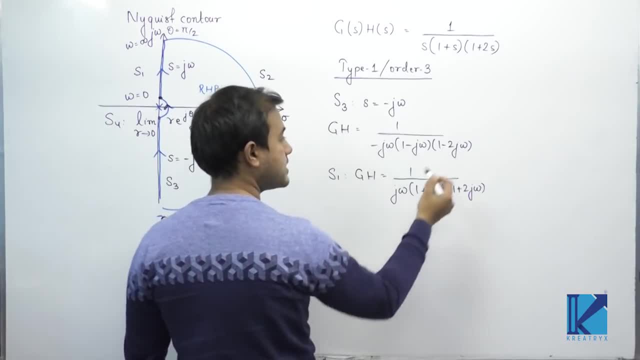 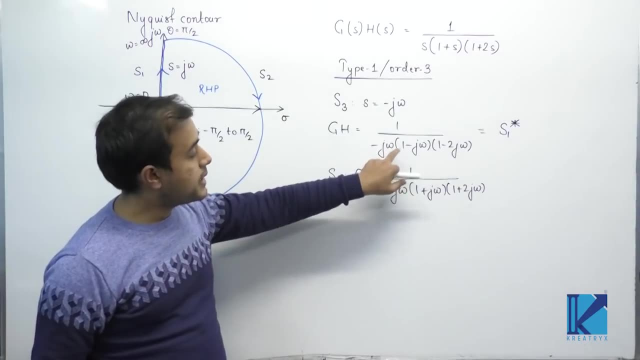 1 plus 2j omega. So can I say this is basically conjugate, for what was there for S1? Here you just have replaced j by minus j. That means we are taking conjugate Graphically. when you take the conjugate of any number. 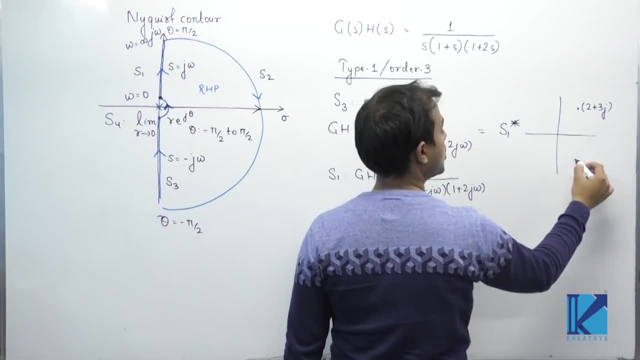 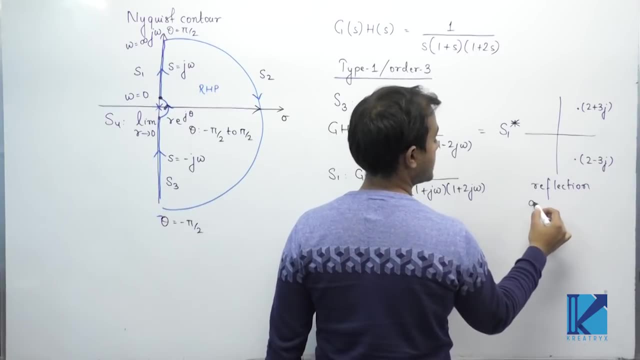 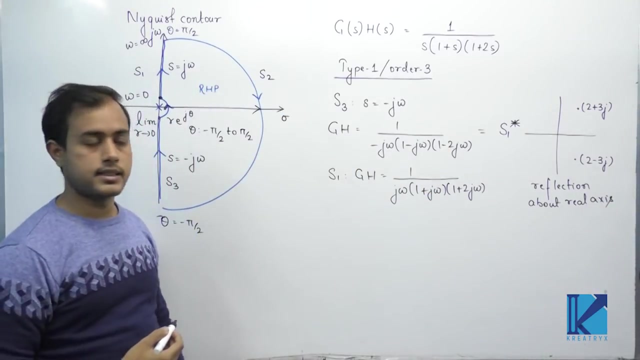 suppose this is 2 plus 3j. If you take its conjugate it will be 2 minus 3j. That is reflection about real axis. So when you take conjugate it is nothing but a reflection about the real axis. 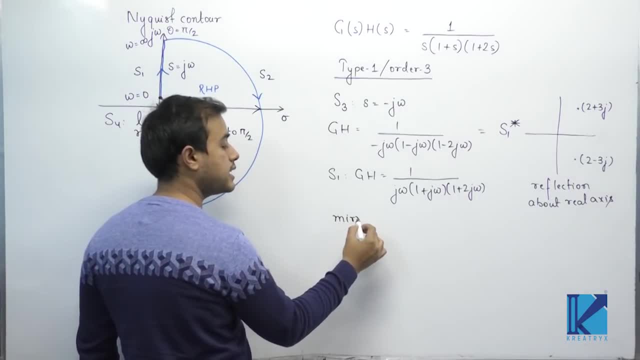 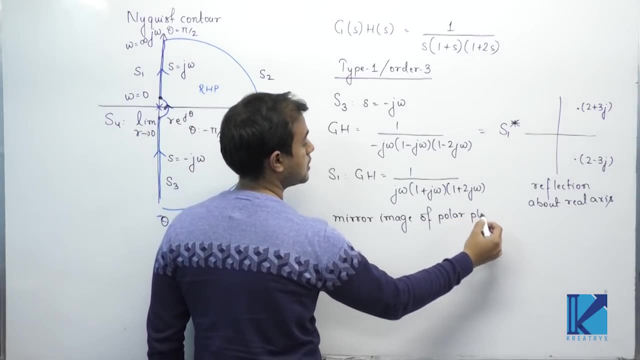 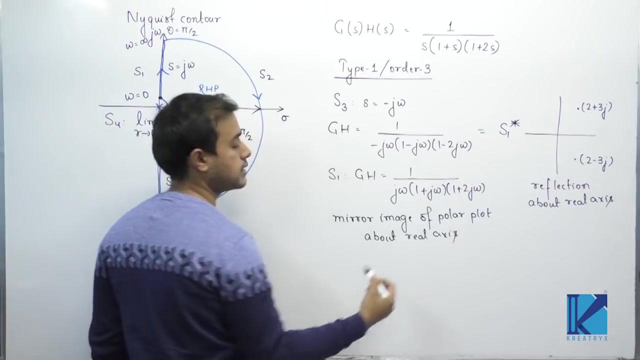 So that means for S3, what we will have is the mirror image of polar plot about real axis. What is meant by polar plot actually here? The curve that we drawn for S1 was also called as the polar plot, So you just have to take the mirror image of that curve. 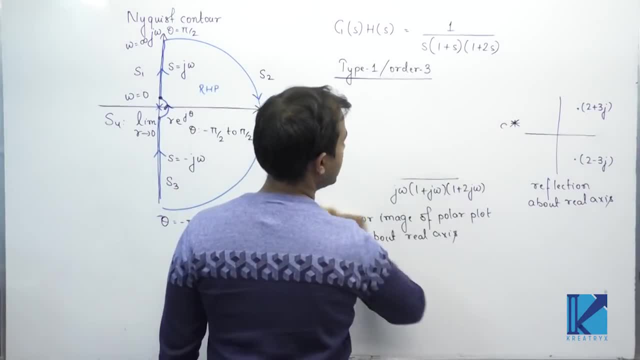 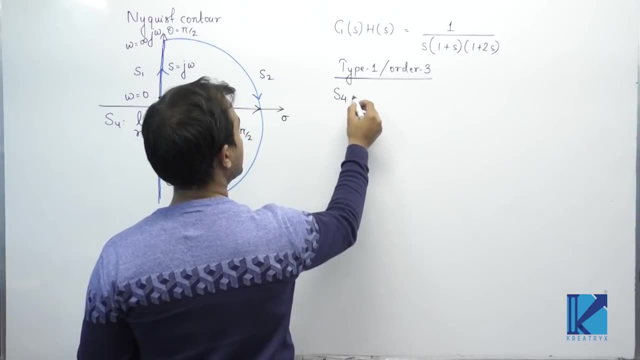 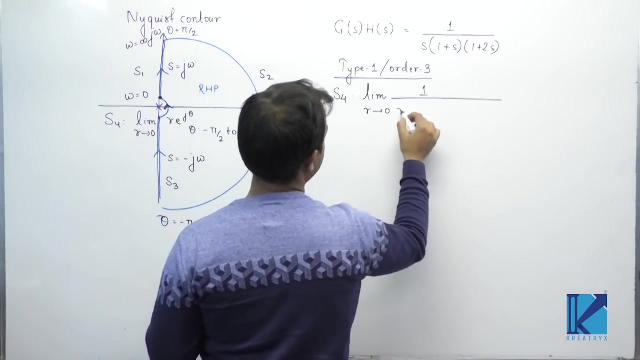 So this is the mirror image of polar plot about real axis. Coming to the last part, that is, S4.. In S4, what will happen? S4? you will take limit in r tending to 0, 1 upon r e to the power j theta. 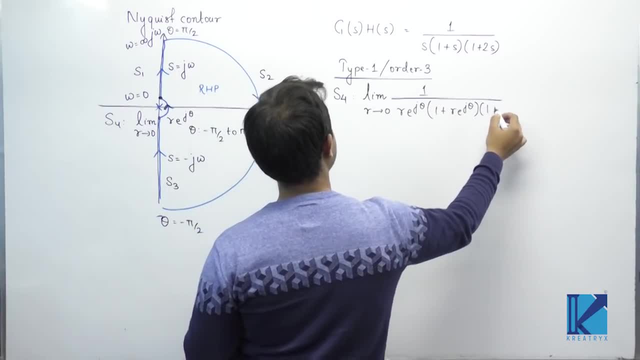 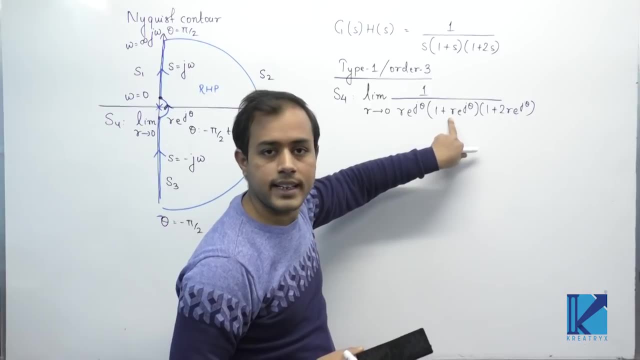 1 plus r e to the power j theta. 1 plus 2r e to the power j theta. Now, if you see this r is very large, It is very less, It is tending to 0.. So in comparison to 1, can you neglect this small term? 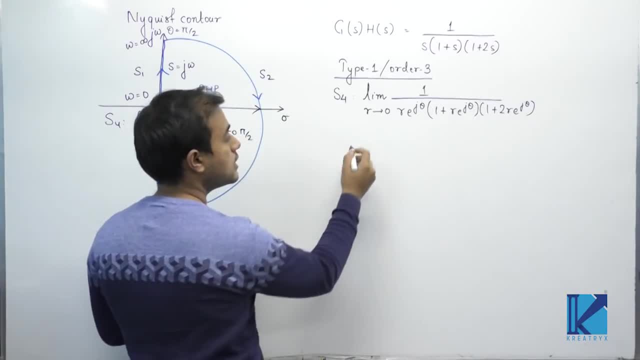 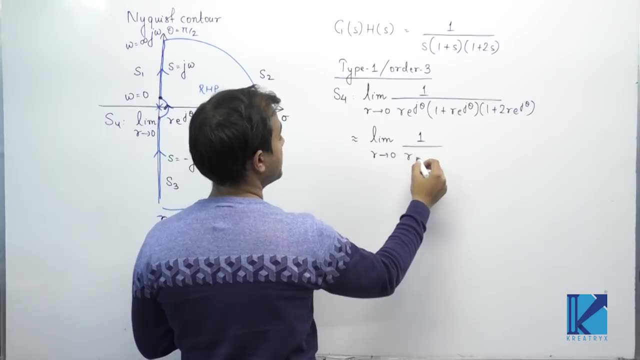 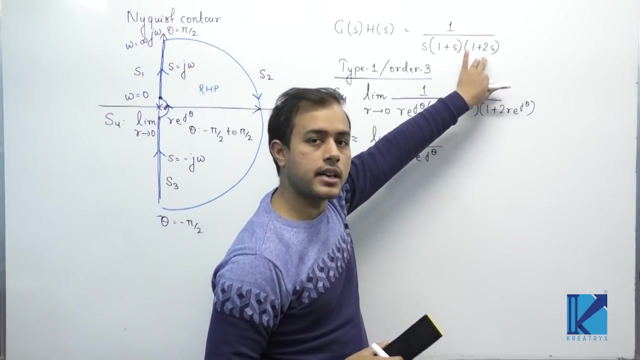 Yes, 1 will be much higher than this term. So this will approximately be limiting r tending to 0, 1 upon r e to the power j theta, That is, all the poles which do not lie at origin will get removed. 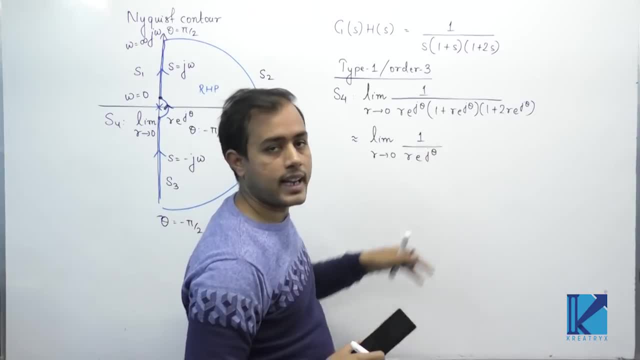 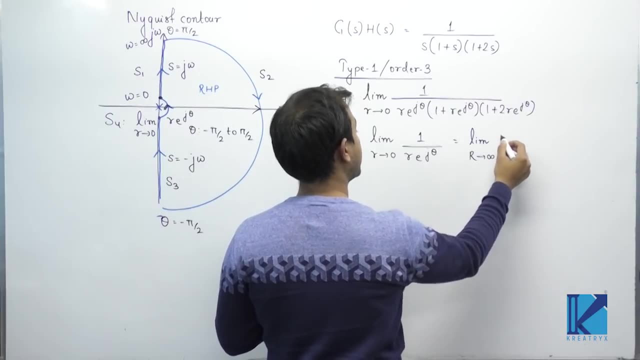 Okay, Only the pole that is remaining is the one lying at origin. So in comparison to 1, can you neglect this small term? Yes, So this will be limiting capital r tending to infinity, r, e to the power minus j theta. 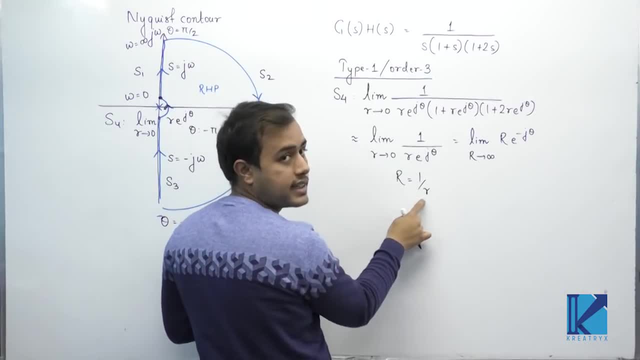 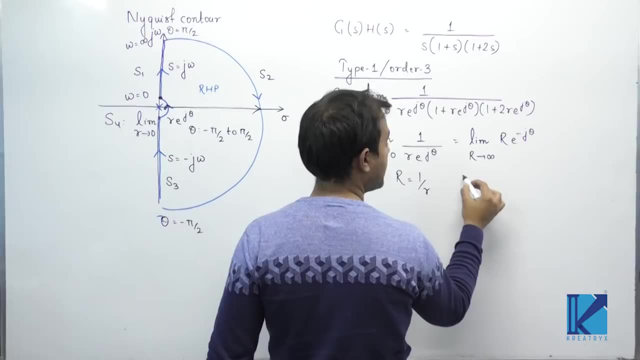 What is this r? It is 1 by r. If this r tends to 0, capital r tends to infinity. And here, since theta was varying from minus pi by 2 to pi by 2, minus theta will vary from pi by 2 to minus pi by 2.. 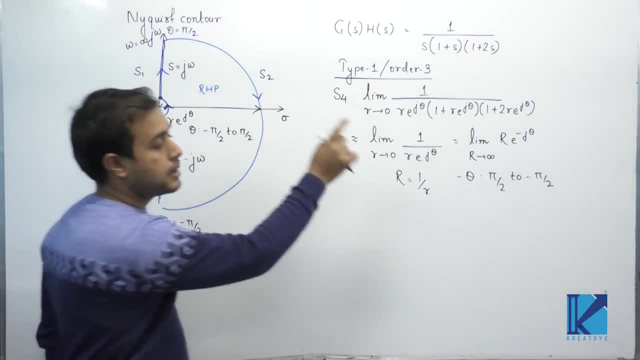 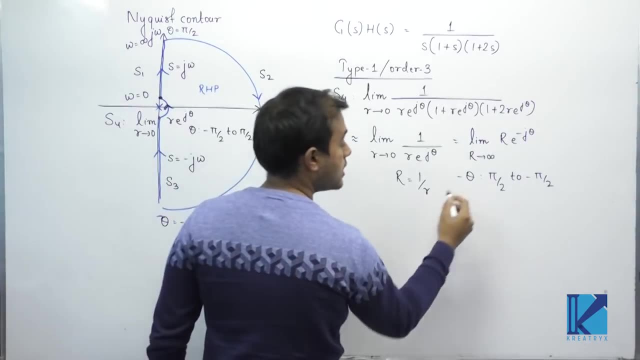 Here theta was varying from minus 90 to plus 90.. Minus theta is varying from minus 90 to plus 90. So minus theta is varying from plus 90 to minus 90.. That is plus 90 to minus 90.. 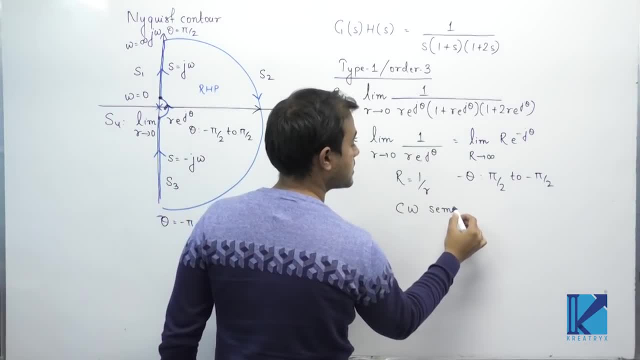 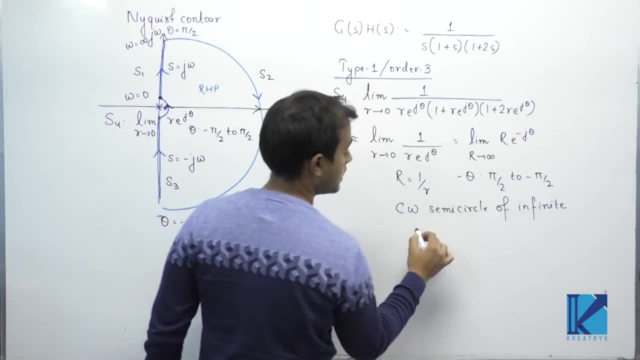 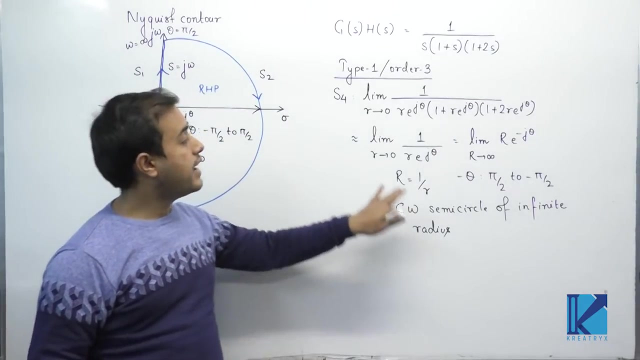 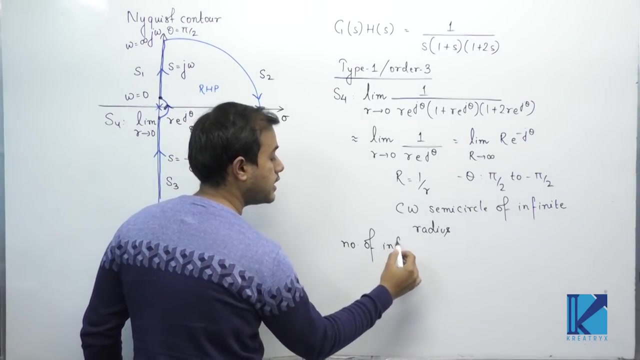 So it will be a clockwise semi-circle of infinite radius. Okay, It will be a clockwise semi-circle of infinite radius, So remember this one as well- Whenever there is a pole at origin. So what I will say: Number of poles, Number of infinite semi-circle equal to type of the system. 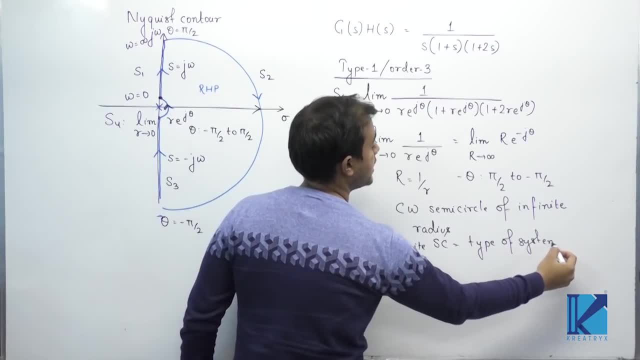 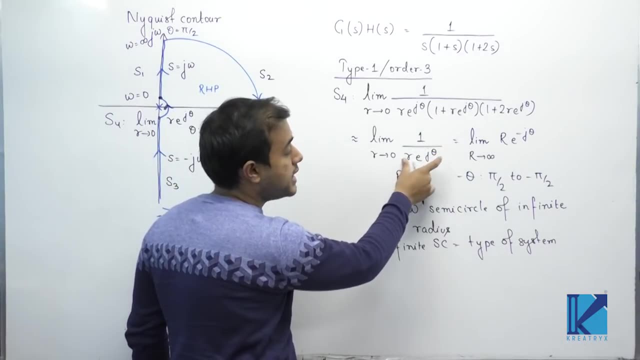 How I am saying this is, as I told you, when you are keeping r tending to 0, the only pole remaining here is the pole that lies at origin, Which means if there were 3 poles at origin, we would have r cubed e to the power j3 theta. 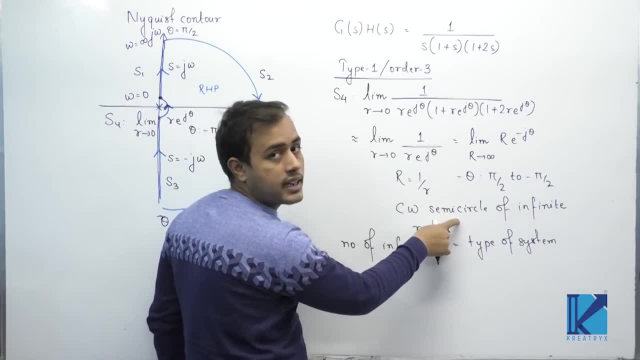 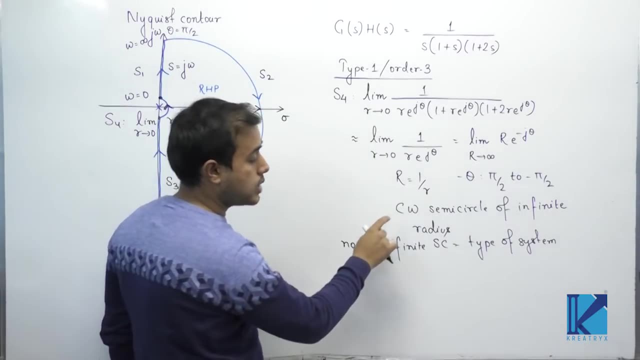 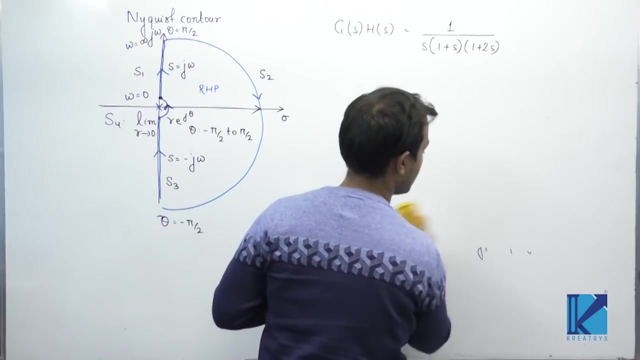 Each pole will contribute one clockwise infinite semi-circle. So number of infinite semi-circle is equal to type of system. Okay, And also, it will always be clockwise. Now, how do I draw the Nyquist plot for this function? Okay, How to draw the Nyquist plot. 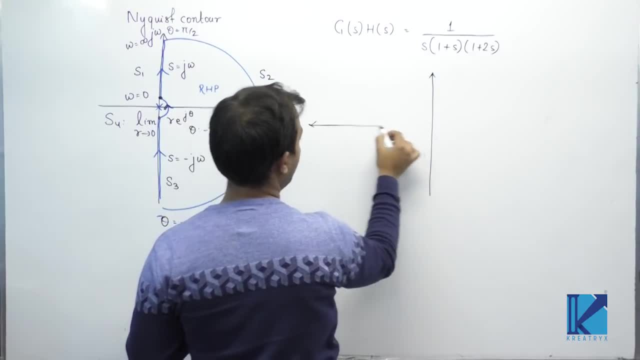 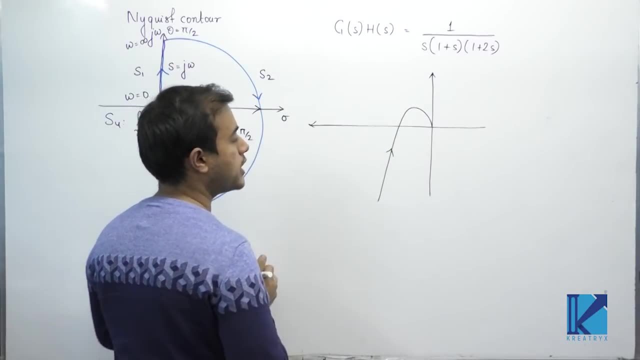 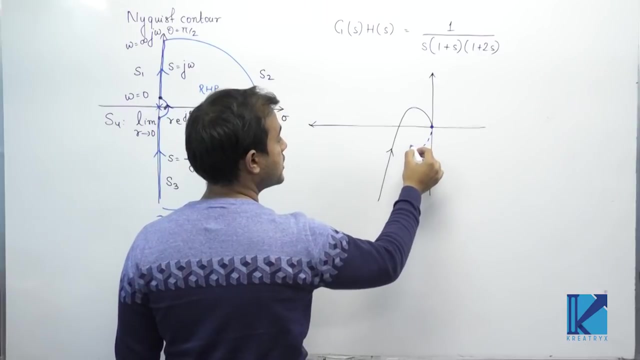 First I will check out the polar plot that I drew for S1.. This one was it For S2, I told you. it will be mapped to origin. S2 is mapped to origin. For S3, I told you, take the mirror image of this curve like this: 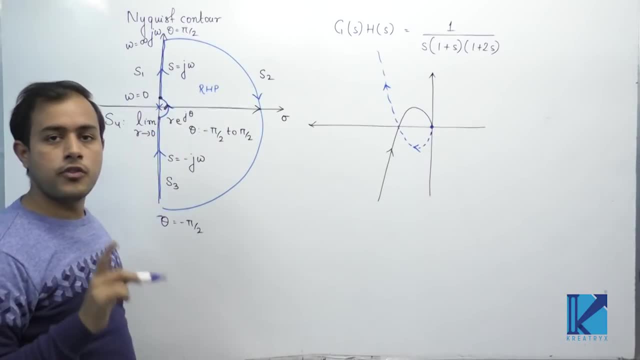 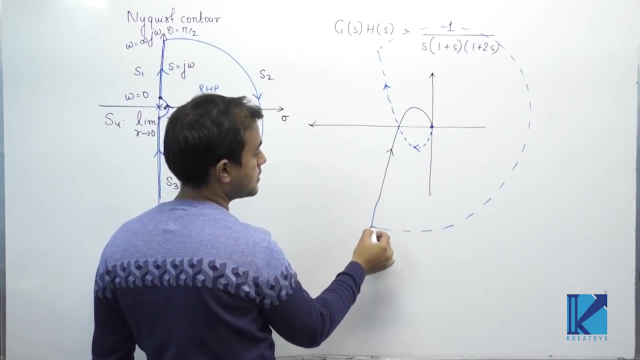 But direction would be opposite. Then I told you one infinite semi-circle, And since the Nyquist plot must be a closed curve, it will go on like this. Okay, Like this. So this will be your Nyquist plot for this transverse function. 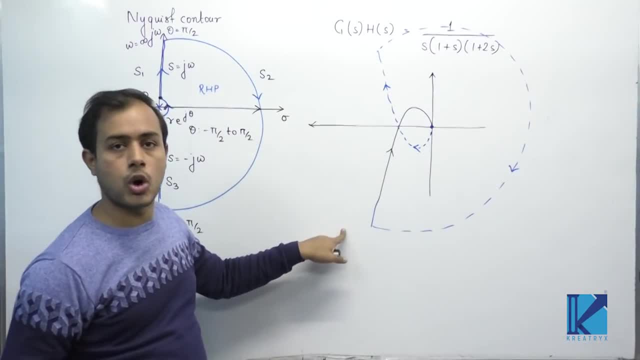 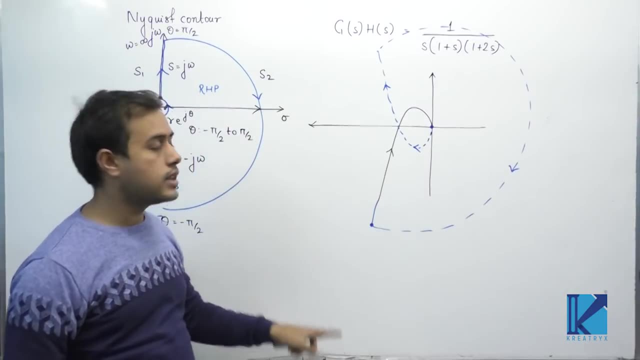 Remember, this infinite semi-circle will always be clockwise And this curve must be a closed curve, That is, it should terminate at the point where it started, because Nyquist contour is always a closed curve. So that is how you can draw the Nyquist plot. 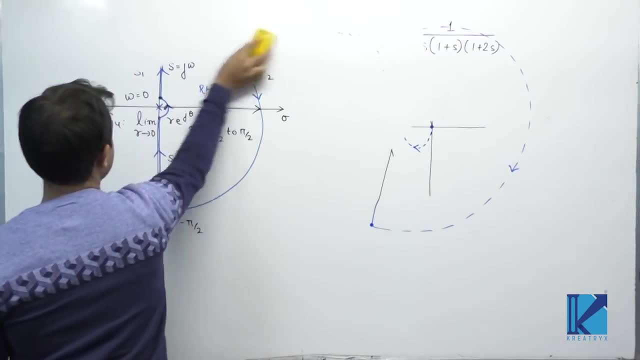 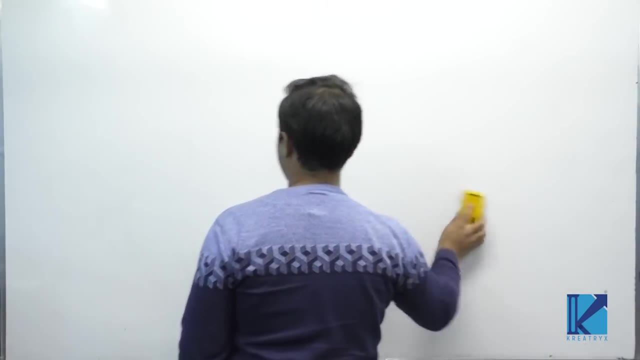 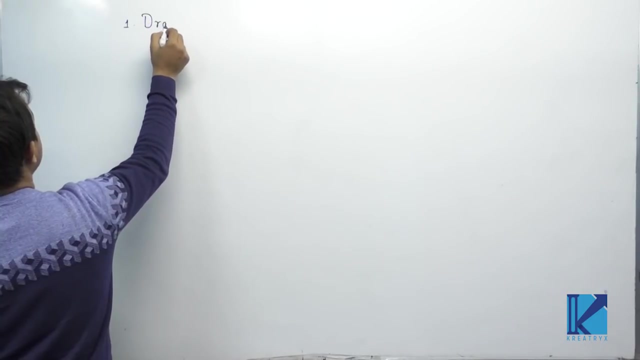 Now let me do one thing, Let me take a more typical example. So first of all, let me tell you the direct trick: How to draw the Nyquist plot directly without considering so many things. First thing, Draw polar plot. That is the plot or the Nyquist plot for S1.. 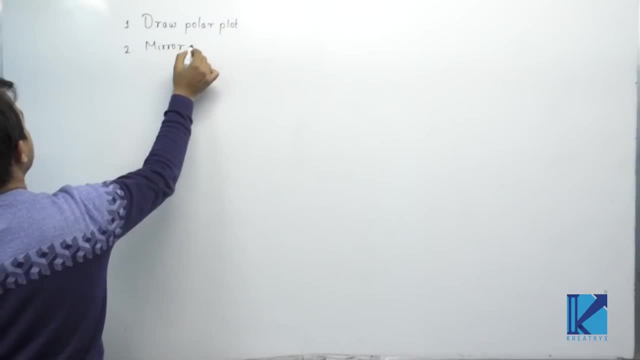 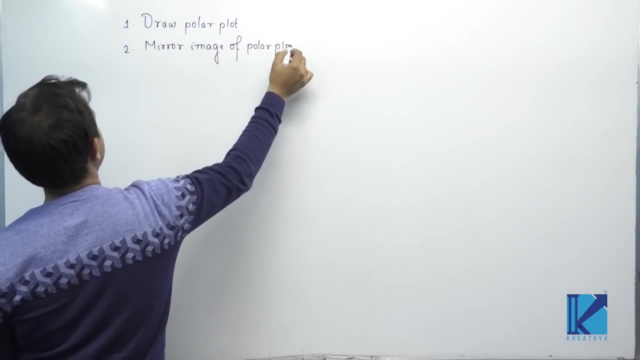 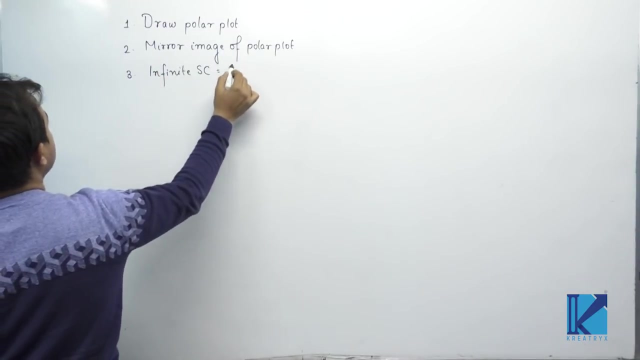 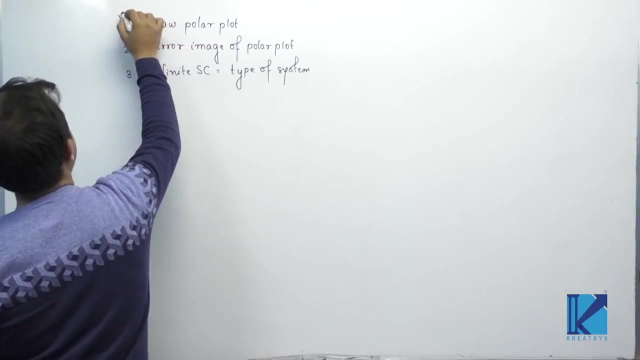 Then mirror image of polar plot. Okay, Then the third one, Infinite semi-circle, which are equal in number to the type of system. This thing you have to draw. The main challenge is only in drawing the polar plot. Is it fine? So let me take an example. 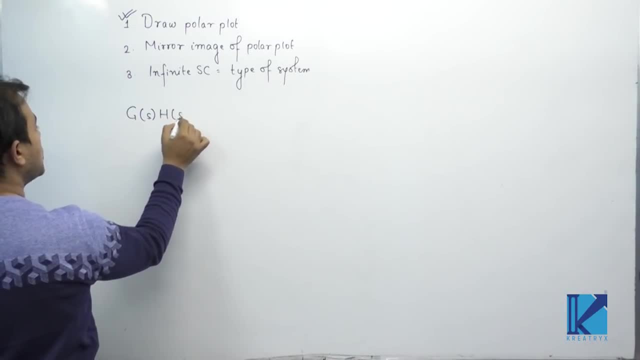 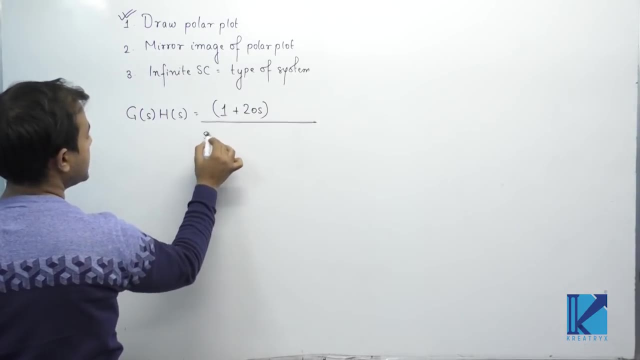 So suppose GSHS is something like this: I have added a 0 as well. Now, whenever there is a 0 in the transfer function while drawing polar plot, what you do is you replace S by GSHS, S by j omega. 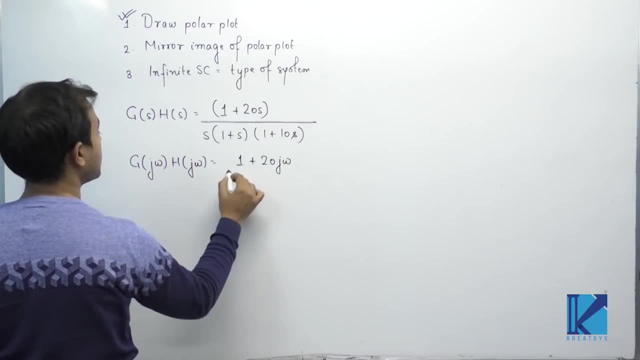 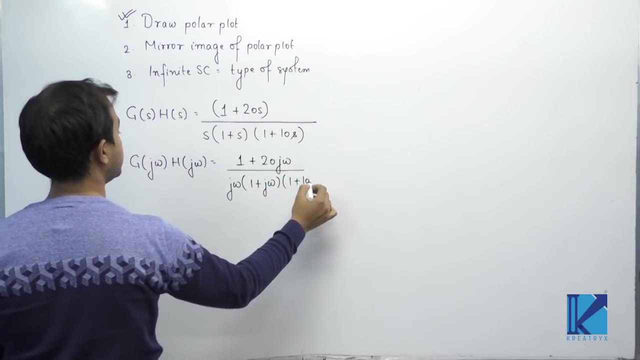 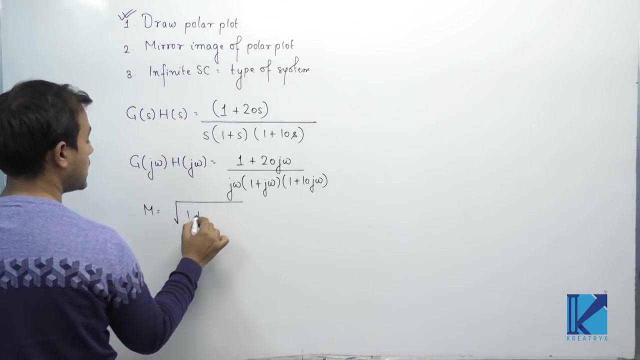 Then what it will become? 1 plus 20 j omega by j omega. 1 plus j omega. 1 plus 10 j omega. Now, in that case, what will be the magnitude Under root? 1 plus 400 omega square. 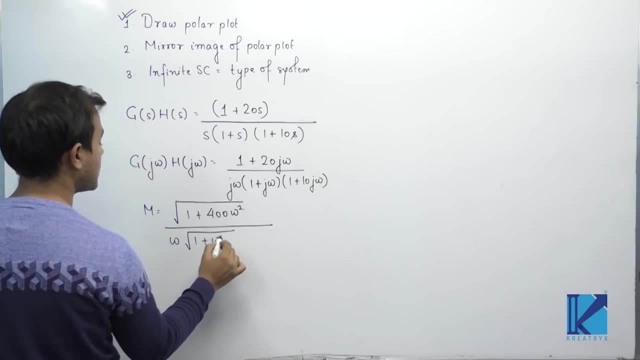 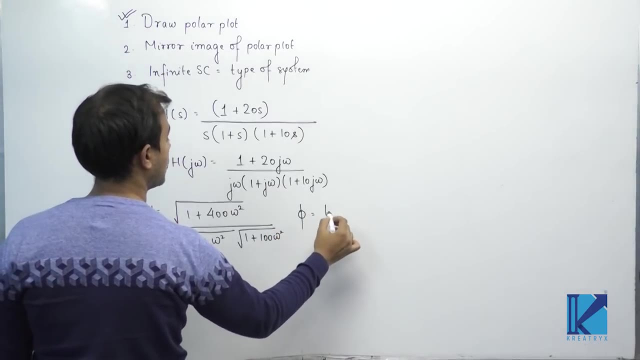 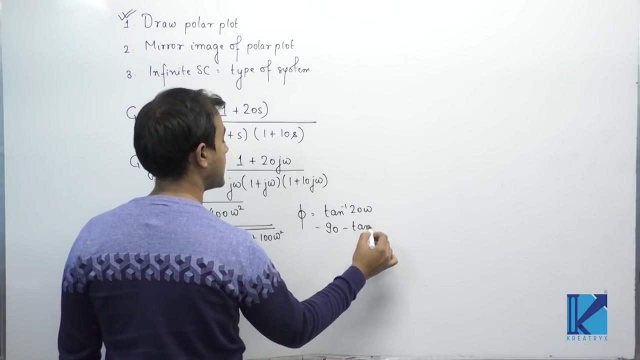 Then omega 1 plus omega square, 1 plus 100 omega square. Then phase For numerator: it will be 10 inverse 20 omega For denominator: minus 90 minus 10 inverse omega minus 10 inverse 10 omega. 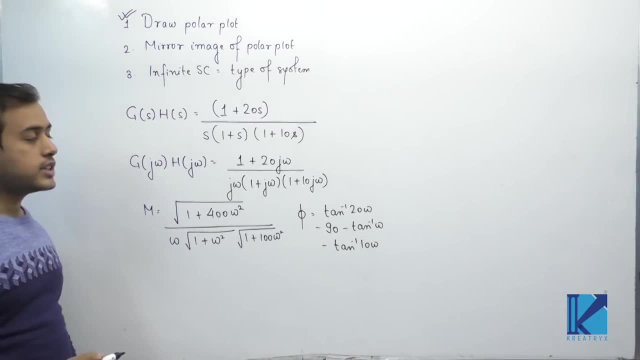 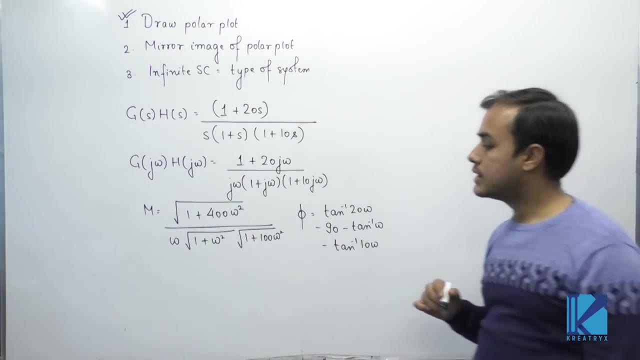 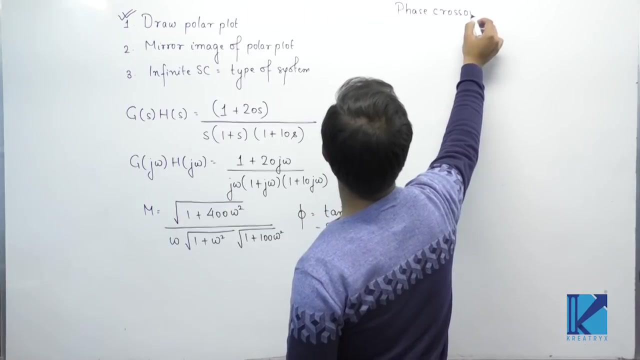 Now as earlier, you can calculate the magnitude and phase at omega equal to 0 and infinity. But in addition to that here you have to find one more thing That is called as the phase crossover frequency, Whenever there are 0s in the transfer function. 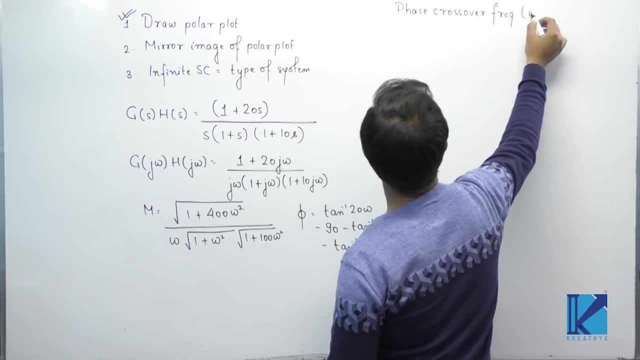 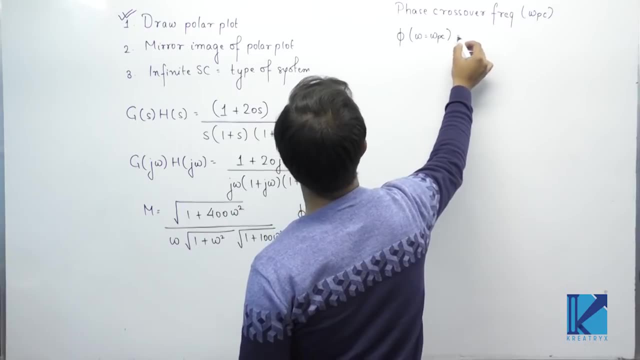 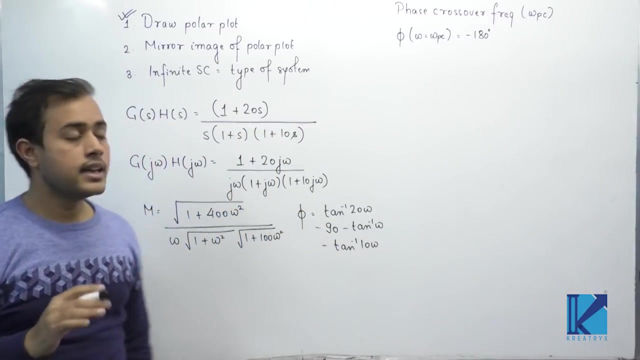 always take care to determine phase crossover frequency, omega pc, That is, the frequency at which the phase becomes minus 180.. Minus 180 means the negative real axis. So why I am doing this is in order to determine the intersection of the polar plot with the negative real axis. 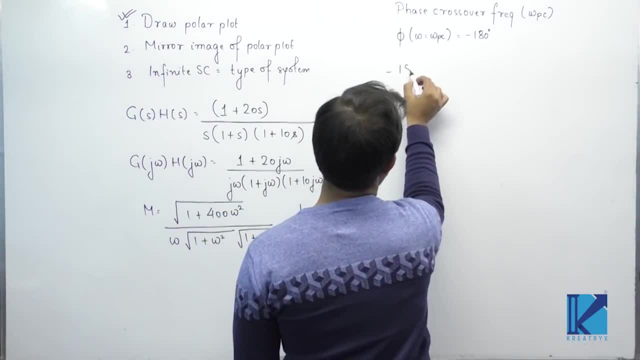 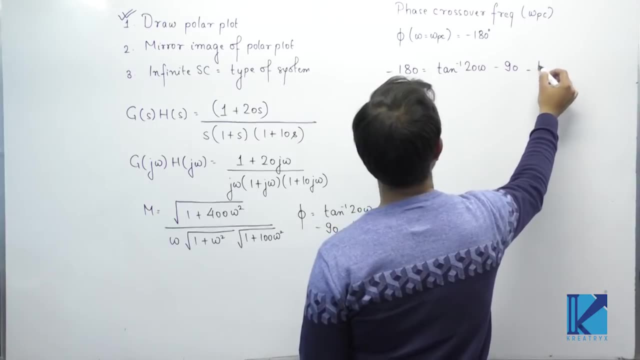 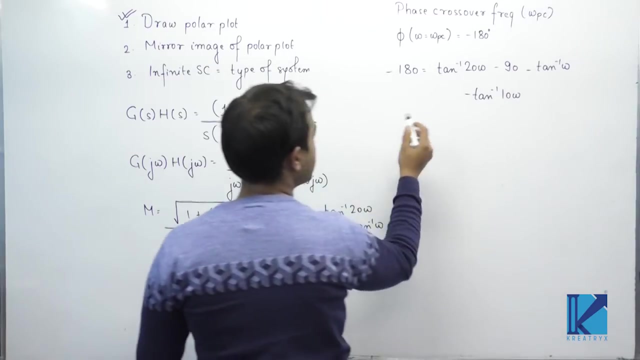 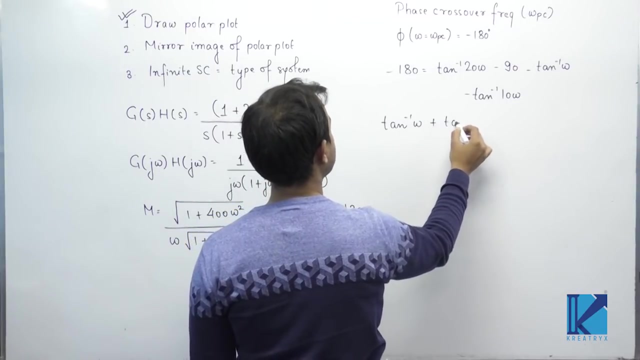 So minus 180 is equal to 10 inverse 20 omega. minus 90 minus 10 inverse omega. minus 10 inverse 10 omega. So take this 10 inverse- last two terms on the right hand side, Sorry, left hand side- 10 inverse omega plus 10 inverse 10 omega is equal to 10 inverse 20 omega. 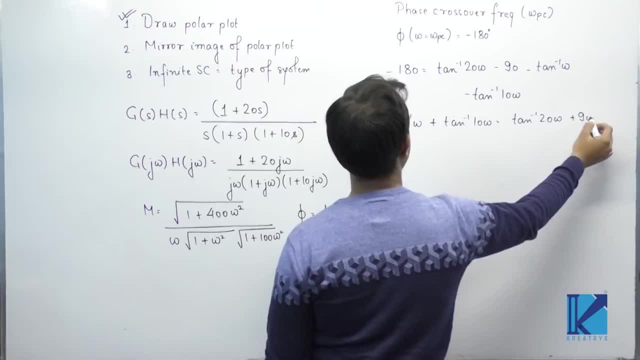 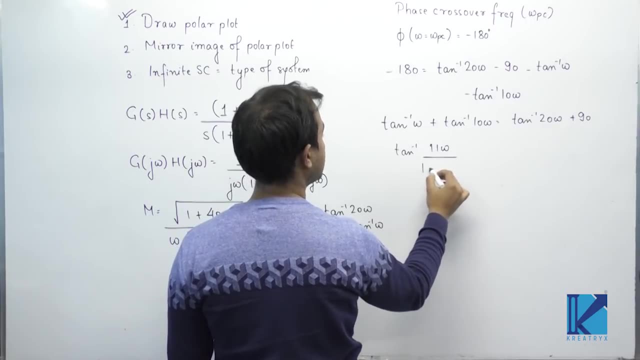 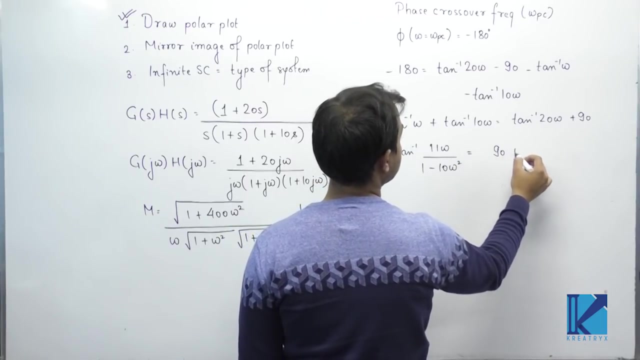 10 inverse 20 omega plus 90.. Take 10 both sides, Or first simplify this: 10 inverse 11 omega. 10 inverse a plus b upon 10 inverse Sorry upon 1 minus a b. 90 plus 10 inverse 20 omega. 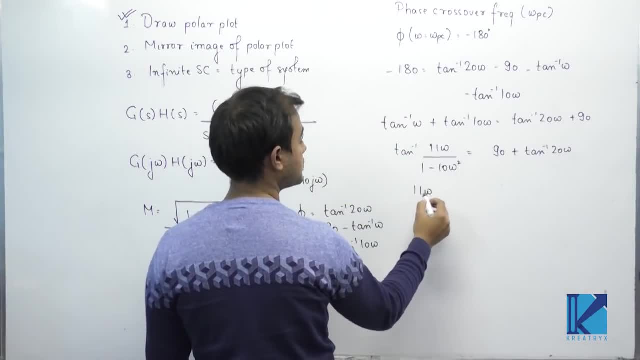 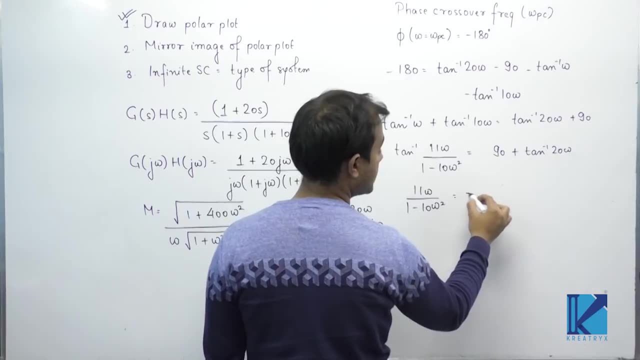 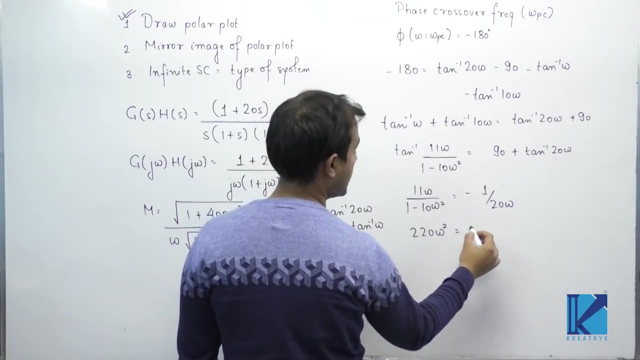 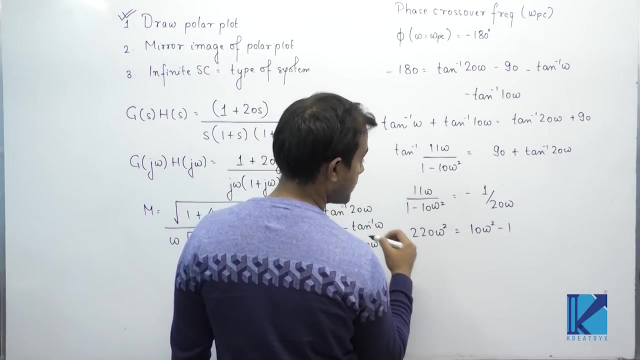 Now take 10 on both the sides. 10 of 90 plus theta is quad theta Minus quad theta. actually So minus 1 by 20 omega, So 220 omega square equal to 10 omega square minus 1.. So how much will this come out to be? 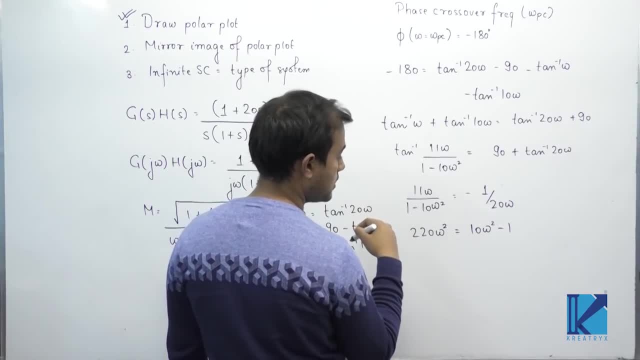 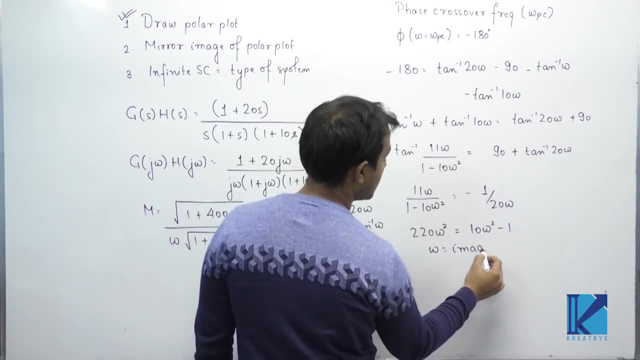 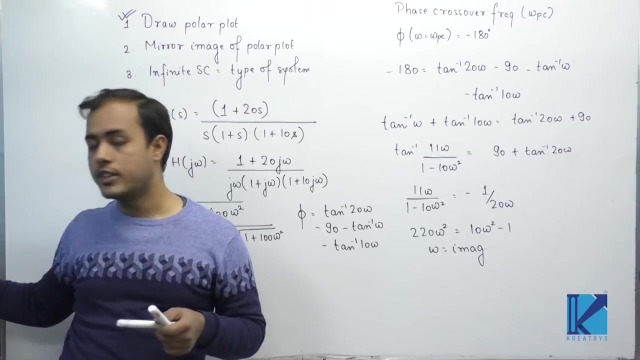 One minute 220 omega square equal to minus 1 plus 10 omega square. It is fine. So now omega will come out to be imaginary, That is, it will not have any phase crossover frequency Or it will not intersect the negative ringle axis. 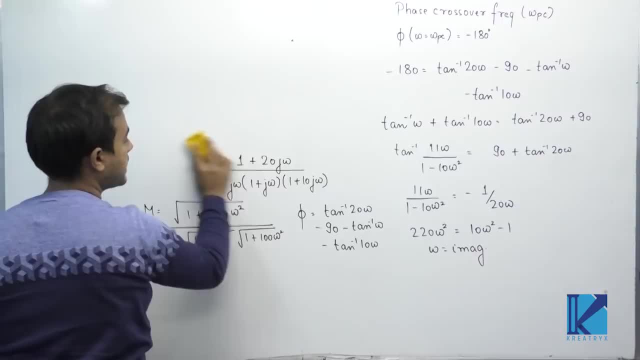 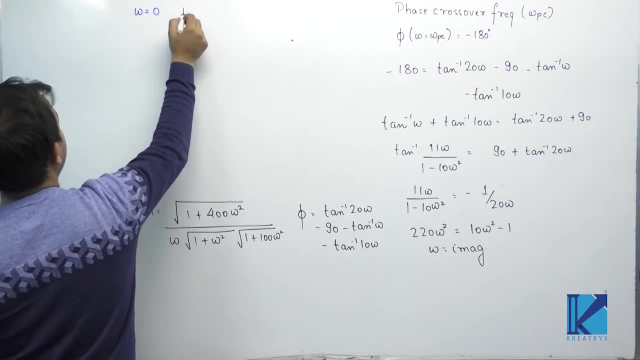 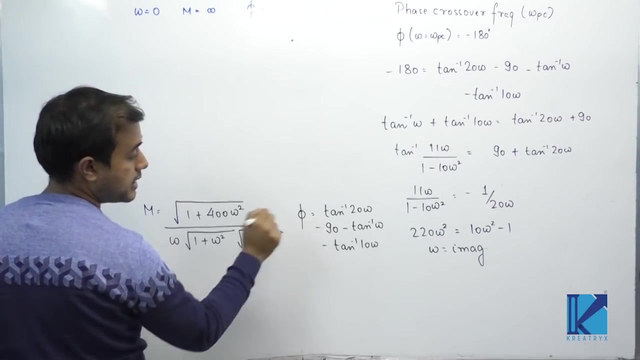 Now what we will do is We will find out the magnitude and phase at 0 and infinite frequency, So at omega equal to 0.. What is the magnitude At 0? it will be infinite. What will be the phase? The phase will be how much? 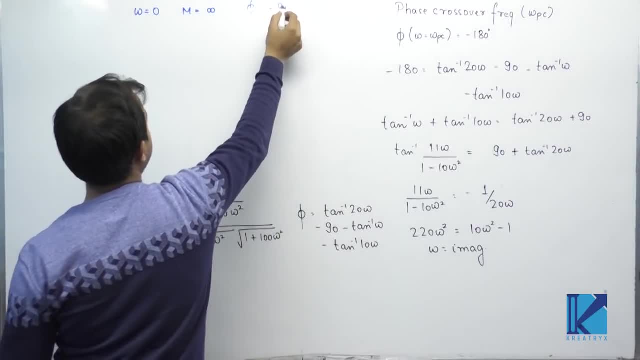 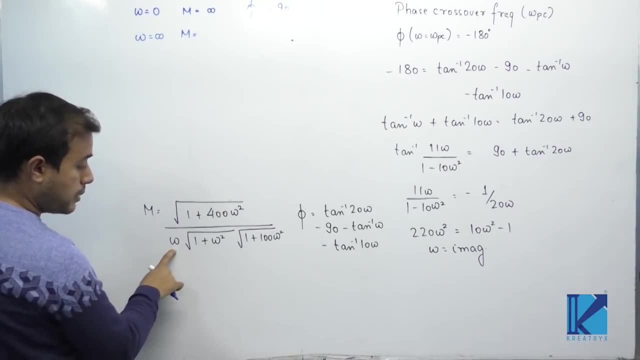 0, 0, 0.. So it will be minus 90.. At omega equal to infinity, what will be the magnitude? At omega equal to infinity, this will become omega. This will become omega because 1 will be ignored. This will become 10 omega. 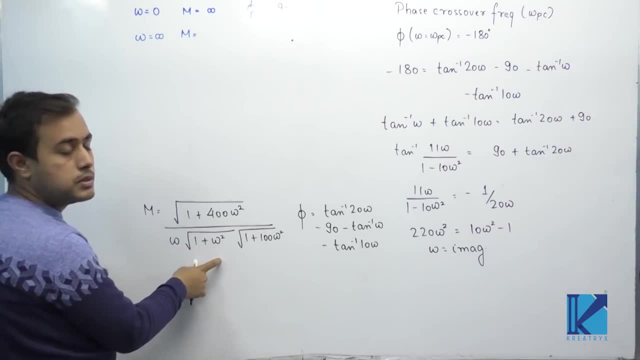 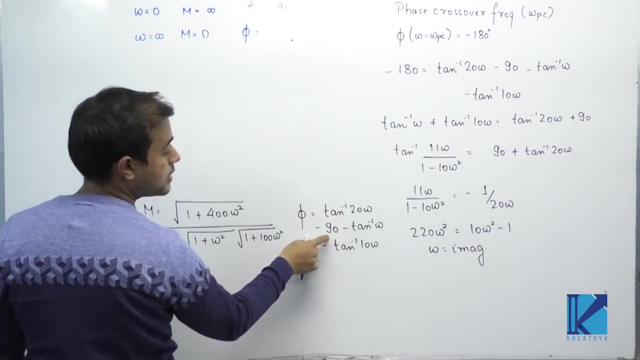 And here it will be 20 omega. So denominator: you have omega, cube, Numerator: you only have omega. So it will be 0.. What about phase 90 minus 90, 0.. Minus 90 minus 90.. That is minus 1.. 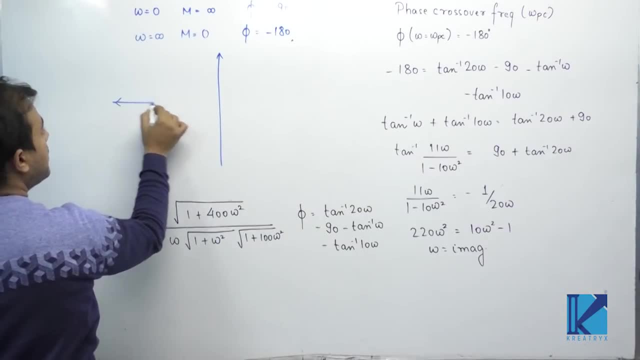 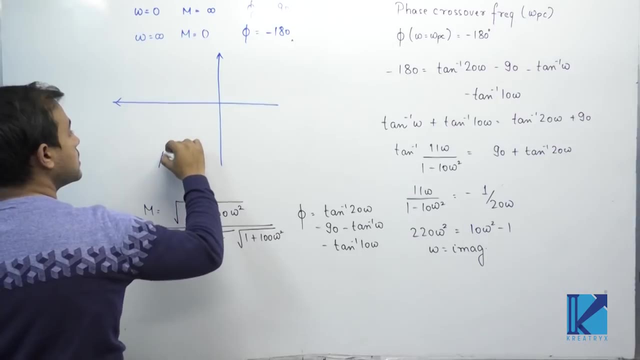 So you have to draw a polar plot. It goes from minus 180. Sorry, minus 90- to minus 180.. Without intersecting the negative ringle axis. So it will be like this. Ok, It does not intersect the negative ringle axis. 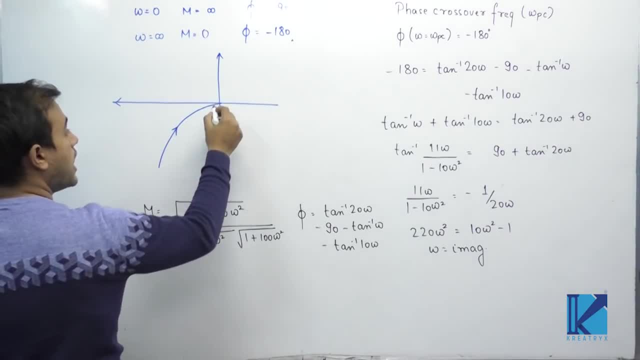 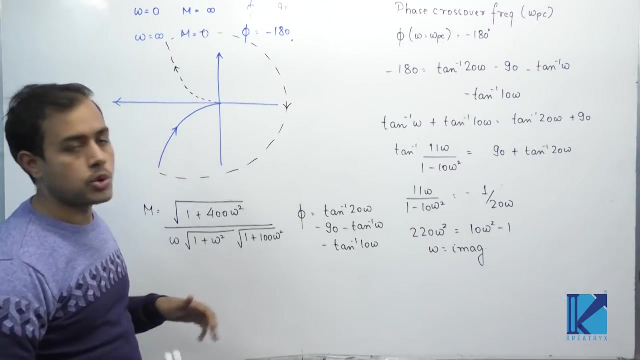 Now You have to draw it's mirror image Like this: Then 1 infinite semicircle, Because the type of the system is 1.. Like this. So this will be the Nyquist plot For this transfer function. So, as I have told you, 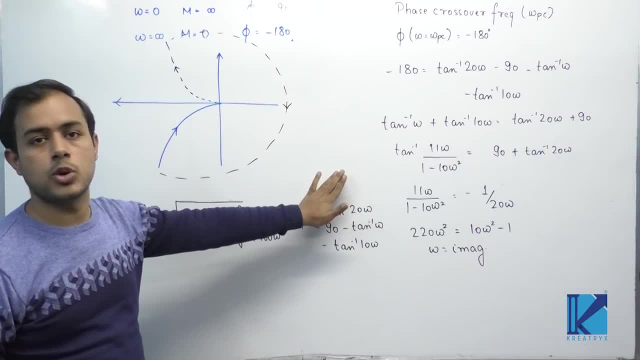 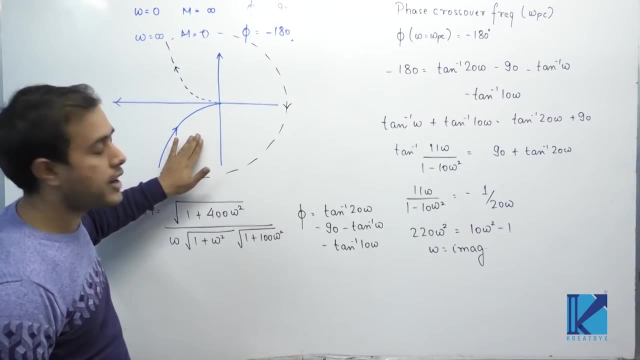 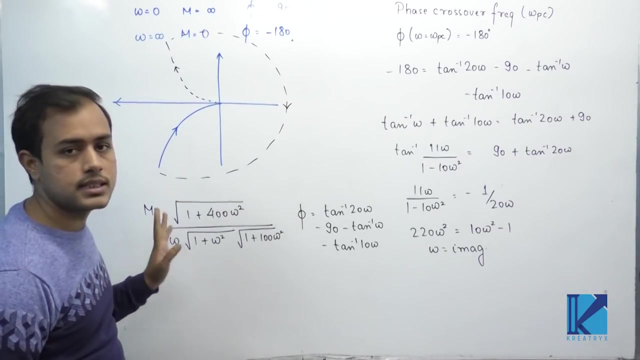 The main challenge only lies in determining the phase crossover frequency In order to understand whether or not it crosses the negative ringle axis. After once you have drawn the polar plot, You can draw it's mirror image And 1 or 2 infinite semicircle based on the type of the system. 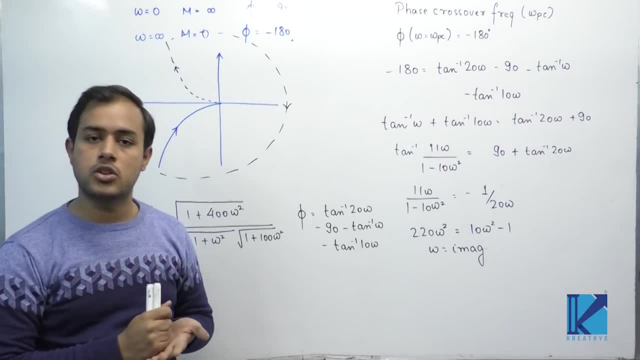 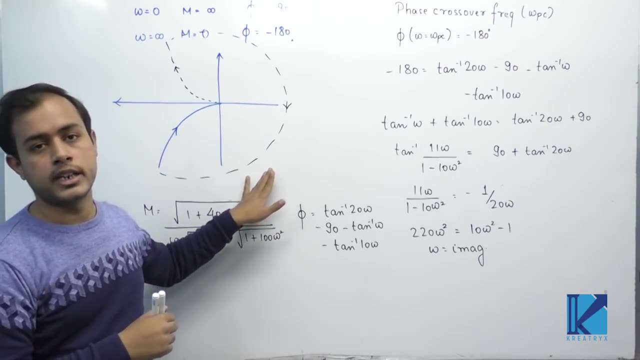 So that is the entire procedure that is involved in drawing the Nyquist plot, And I have explained in one more video that I posted earlier How to use this Nyquist plot in order to determine the stability. So I have explained you Nyquist stability criteria as well as the Nyquist plot.